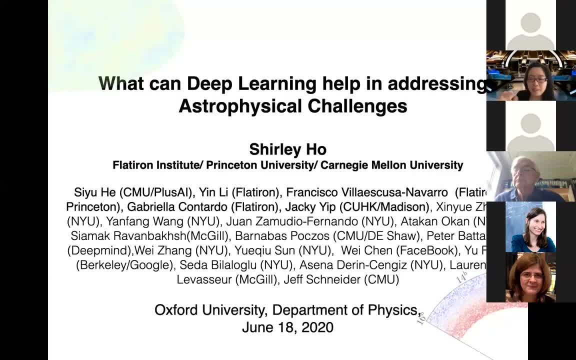 Hi everyone. Let me just say hi to everybody and thank you for inviting me here. Can you guys hear, okay, or see the title screen? okay, I think someone's speaking, but can't It's muted. Yeah, yeah, Fine. 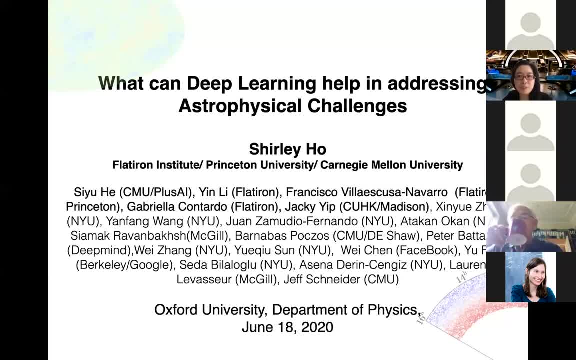 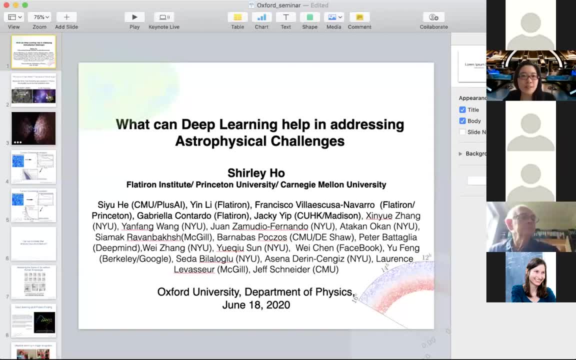 Okay good, Can everyone sort of see everything? more or less okay, And I would like to encourage people to basically sort of shout out questions. I won't be able to moderate while I'm giving you questions. I'm just giving the talk because it's the way the Zoom is: When you're sharing the slides, you don't get to see all the participants so easily. 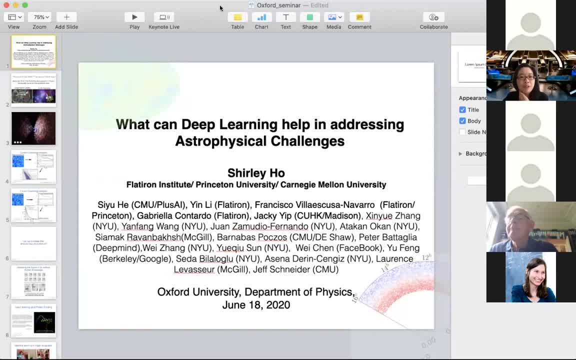 So people just should feel free to shout out questions anytime. I will try to pause, you know, at certain parts, when we finish certain sections about the talk for questions also, but just feel free to yell out questions. I was one of those people who were trained by. I don't know if any one of you know Gerald Stryker very well, but you know he tends to ask questions very loudly. 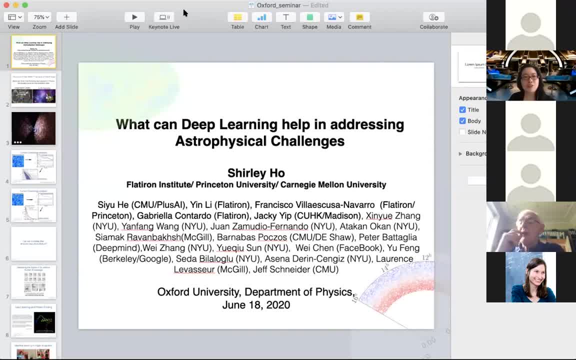 And I was a good student. I was a good student in Princeton when he was very active, So we're very well trained to answer random questions at random points, And so just don't be shy. Okay, And let me try to start. 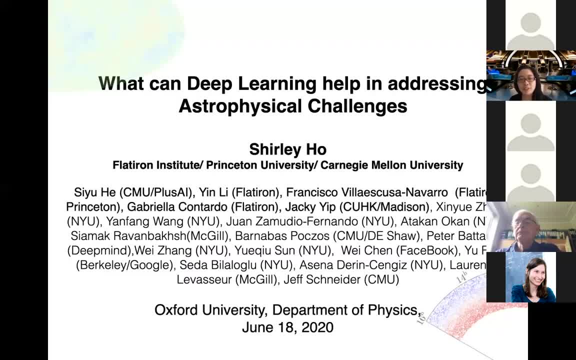 Okay, so today I'm going to talk about what can deep learning help in addressing astrophysical challenges? I'm Shirley Ho, I'm currently at the Flaherty Institute as a group leader And I also have joint appointments at Princeton, and also I'm an associate professor. 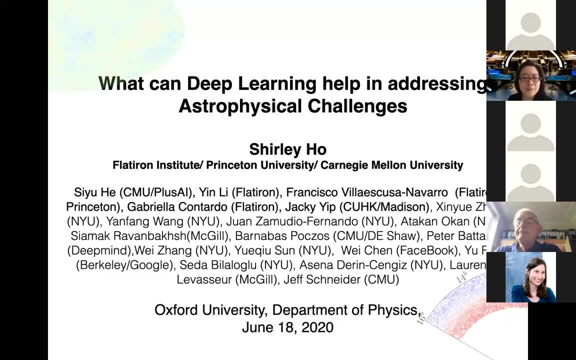 And with this adjunct position at Carnegie Mellon, still where I was tenured at Carnegie Mellon before I moved to Berkeley and then Flatiron. You might wonder why you move so much, but I guess just opportunities called when Flatiron Institute was first set up. 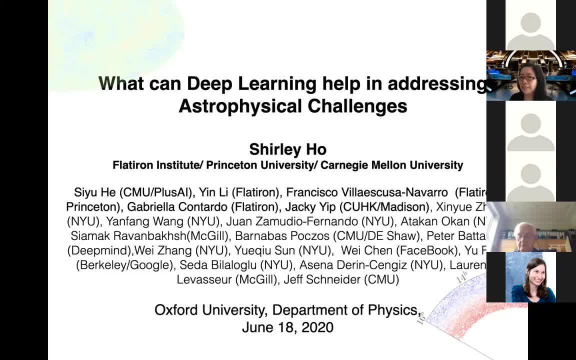 Do anyone know about Flatiron Institute in this group? Yes, no, I can't see your heads for sure, because I need to. A lot of people are not having videos up. No comments, don't be shy. You can also press space to unmute, just momentarily. 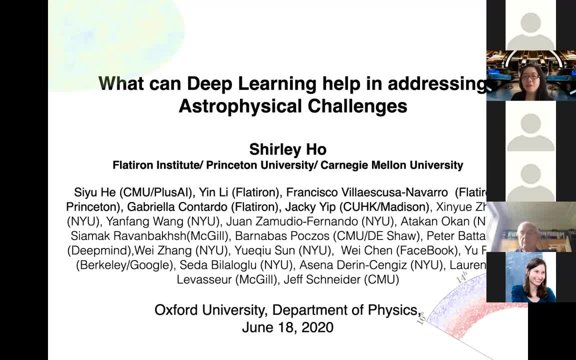 Some of us are familiar with Flatiron, I think. Okay, I'll just quickly say a few things. I've been in the Institute for about two years And before that it was basically an idea. It really was born out of an idea. A group of us went to Jim Simons and said it would be really cool if we combine, you know, these computational tools that people 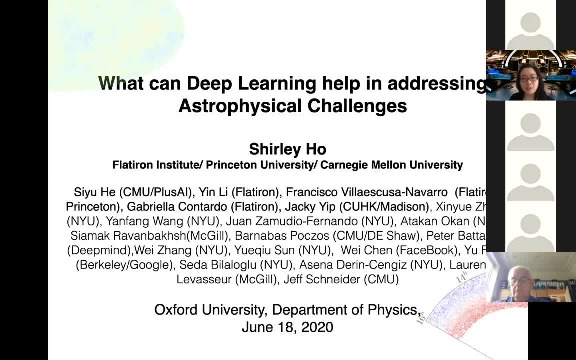 wanted or are developing and all the astrophysical and other challenges. You know, Flatiron Institute has four, actually now five different centers: Computational astrophysics, computational biology, the computational quantum systems and computational for mathematics. And the newest one is for neuroscience. 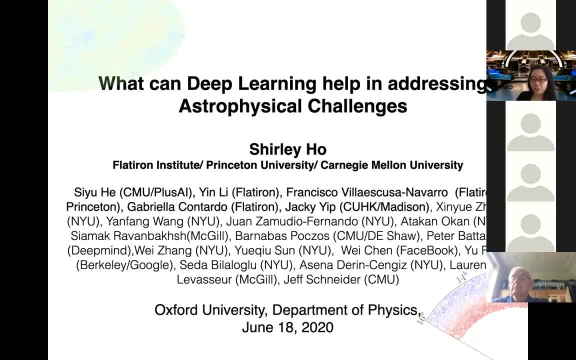 So a lot of these topics have challenges that could be possibly addressed by having more computational methods involved. And for CCA you know the computational methods, not only just deep learning or other things like or like data science, but also simulations. you know numerical simulations, very heavy on that side too. 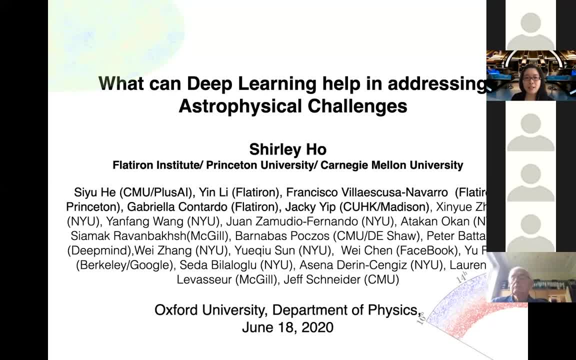 And so that's why I was called and asked: you know what do you want? to become a group leader, to lead the group. You can name whatever group you want. It was kind of funny- And to look at how to apply the tools such as data science, tools that we're developing very rapidly, such as deep learning, to you know, astrophysics problems and challenges. 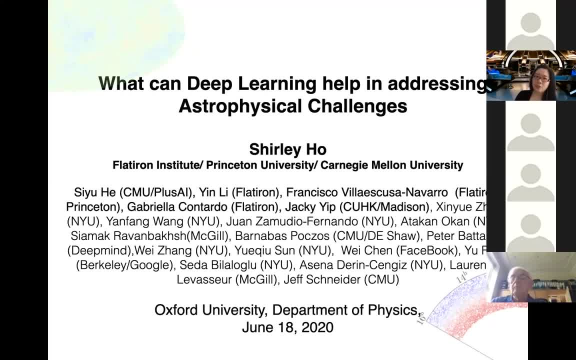 So that's why I moved from sunny California to New York, which recently has become the headline in many different countries, I guess because of COVID-19.. Alright, so that's the backstory. The work here I'm going to present are not possible without all these postdocs and students. 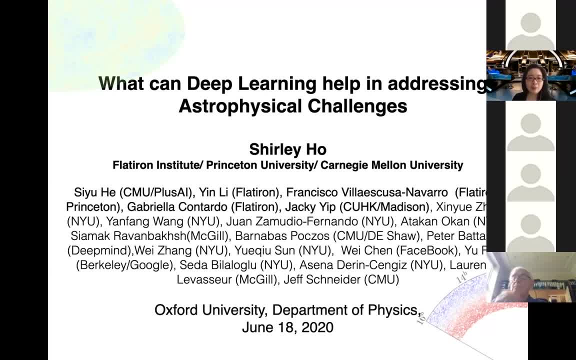 The work here I'm going to present are not possible without all these postdocs and students. The work here I'm going to present are not possible without all these postdocs and students And my collaborators. I highlighted some of the postdocs here And the students here specifically did a lot of heavy lifting. 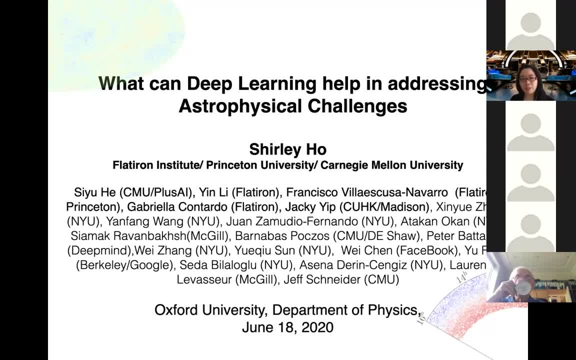 Siyu He, who has now moved to plus AI- She was my Carnegie Mellon student- moved me to Berkeley, then Flatiron, Actually now graduated and now happily working at the AI industry making self-driving cars. actually, Ying Li, who is at Flatiron, who is a postdoc at Flatiron- 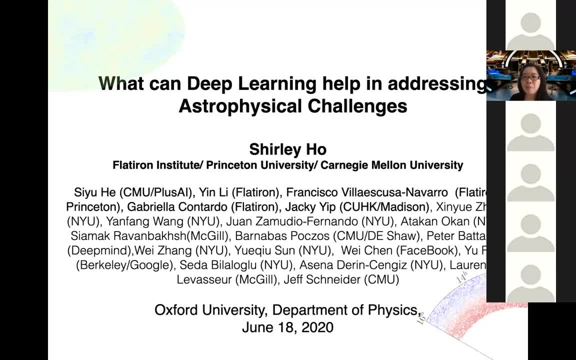 Pat Koh, Francisco Felicista Navarro, Tricia Moffo at Flatiron and Princeton. Now just moved to Princeton Western, to Princeton. recently Gabriela Contardo at Flat End. She's basically a complete machine learner but recently has been, I guess, converted to astrophysics and machine learning. Jackie was an 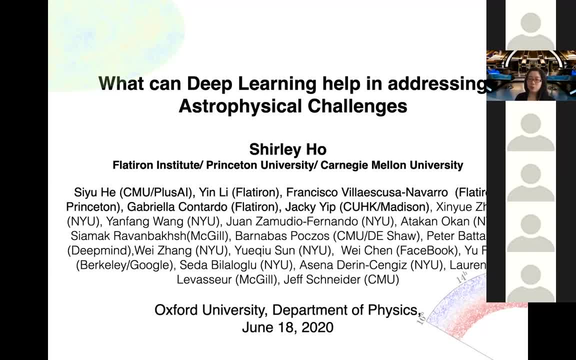 actually intern at summer from CUHK, which is Chinese University of Hong Kong, and he's moving to University of Wisconsin-Madison for grad school in the fall. And there's a bunch of NYU students here who did a lot of heavy lifting for one of the projects The master students were. 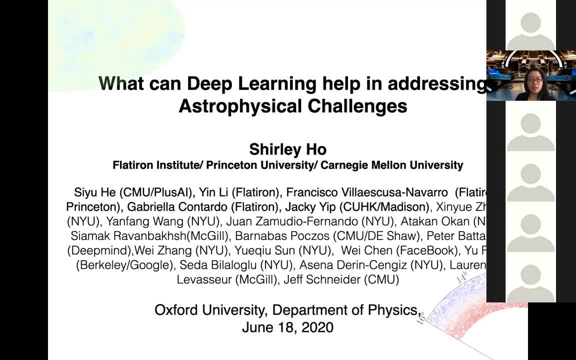 Center for Data Science, and Simon Reffenbach and Barnabas Postle, Peter Vitegli and Jeff Schneider are all machine learners from you know, CMU, McGill and DeepMind that we work heavily with, And, yes, so this is not possible without the students. Without further ado, let me just talk. 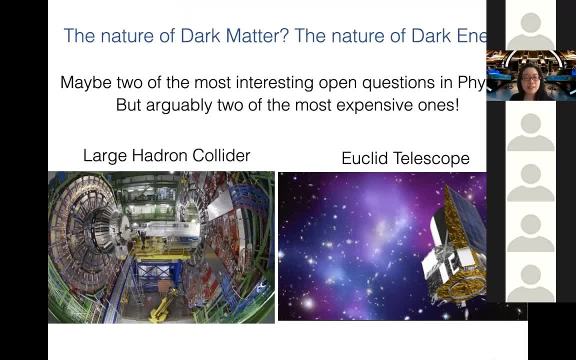 about the work. So with this crew, I guess I don't have to explain why we care about the nature of dark matter or the nature of dark energy, that they might be the most too expensive to do, but I think that there's a lot of interesting open questions in physics I mean. 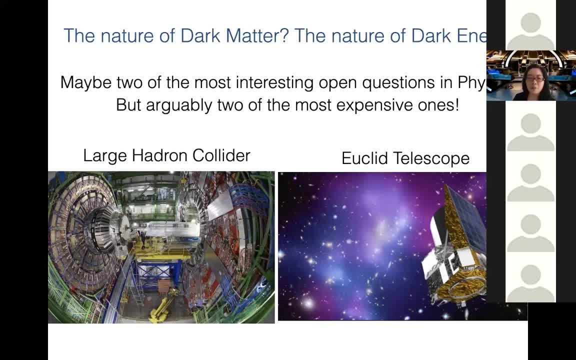 the synonymous cells you probably just heard recently got people very excited and I would love to hear what people think about the synonymous cells that just came out afterwards. And in this you know, I see, and of course in Europe, this huge amount of work in Euclid also. 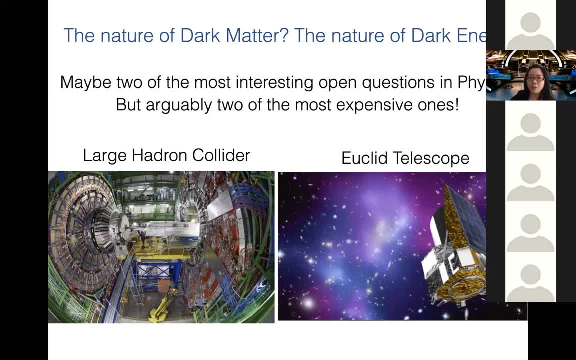 they're all costing possibly a lot. I mean, maybe you don't agree that the two most important or interesting questions in physics are open, but arguably two of the most expensive one, I would say, are the ones that are the most expensive and the ones that are the most expensive. 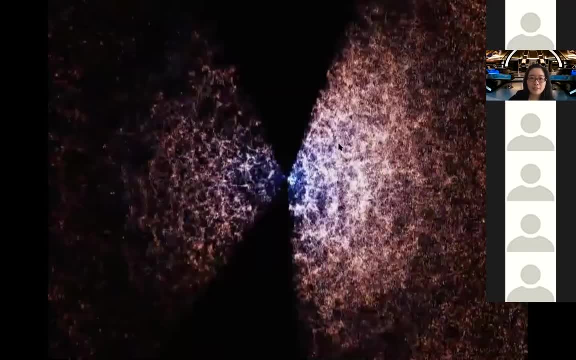 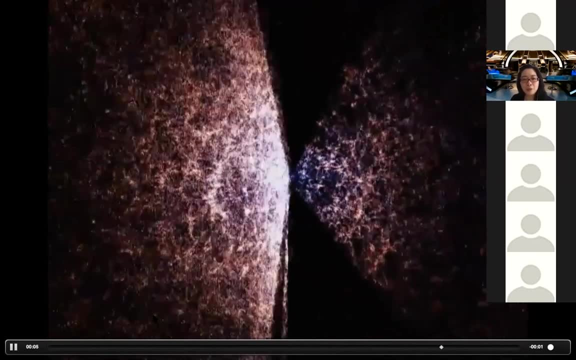 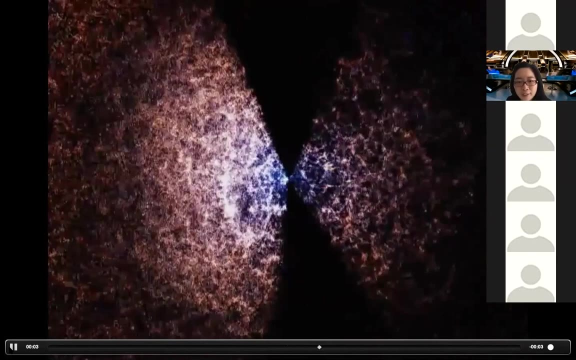 So I'm going to give you a couple of questions. So what do you take all this money, build these telescopes. what do you get? You get, basically an observation of the universe. Here is actually a true, real universe observed by Sloan Digital Sky Survey, and it was every single dot. here is a 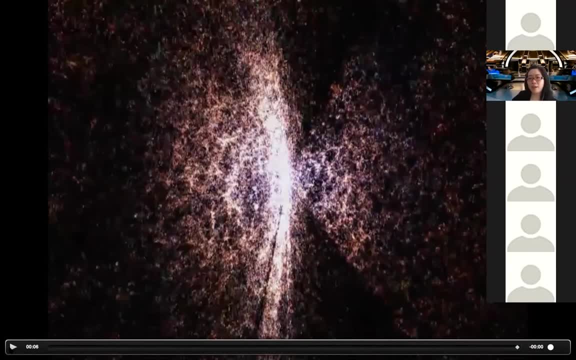 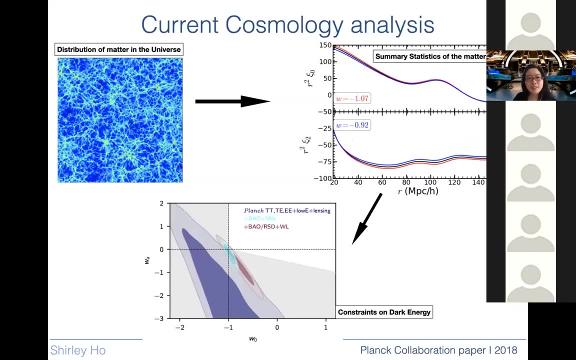 galaxy observed by Sloan and you can see this large-scale structure map in the video and you say, oh, this is the universe. And traditionally that's what we do. We take this cosmic web, this distribution of matter in the universe, you plug it into some kind of pipeline. but 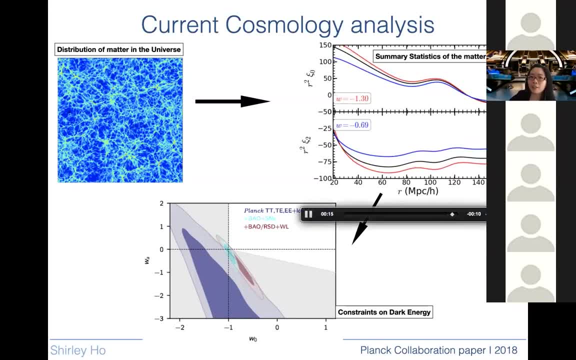 you know, really just some statistics of the matter field, or the galaxy field. We call it the correlation function on the right-hand side, and I'll click this and it will go And, as you can see, that, when you change the dark energy equation of state, which is basically a, 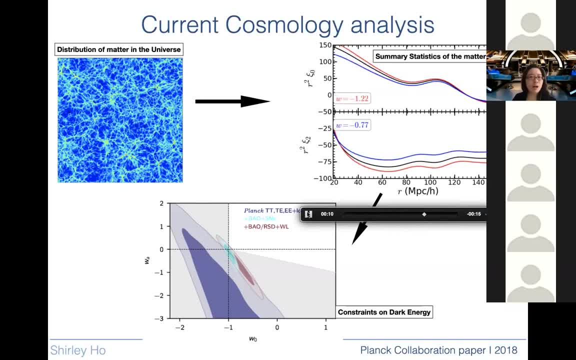 ratio between pressure and density. unknown object or substance, whatever you want to call them, probably substance, and you will see that the correlation function in the monopole on top and the quadruple in the bottom change. This is just observed. some statistics of the matter field. 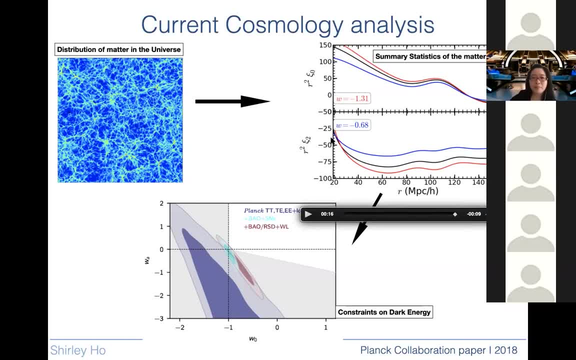 People tend to take the field on the left and compress it to the right, and then you'll compare it to the theoretical expectations and you'll get a constraint on the dark energy. here You can probably see, this is Planck 2018,. 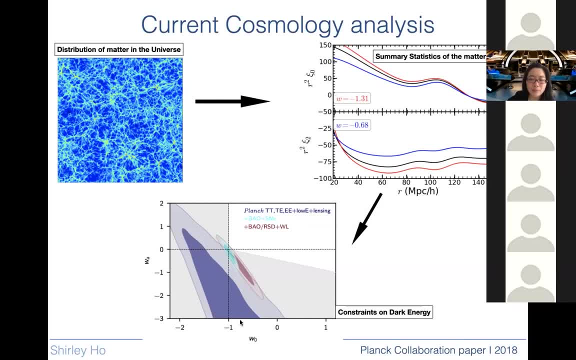 and this is Planck 2018, and this is Planck 2018.. paper where, if you take Planck, you get NTTT, all the lensing stuff from CNB. you get this. This is the different parametrization of the dark energy. You can see WA. 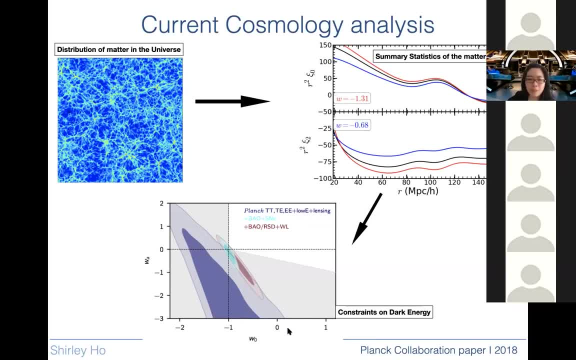 W0 for the experts here, but it's just one of the many parametrizations that people like to use to describe dark energy, sort of like a Taylor expansion. And then you can see that if you add BAO, which is basically from larger structure, and RSD and weak lensing, these are all from the 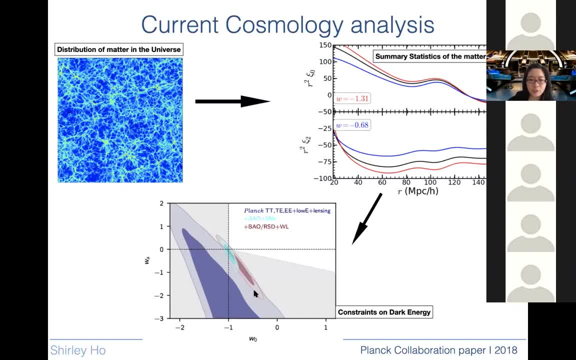 cosmic web, which is the brown here you can see this is shrunk dramatically. And if you add also supernova plus BAO, you shrunk even more in terms of constraints on dark energy. Similar things happen when you look at other things such as the neutrino masses. Here we 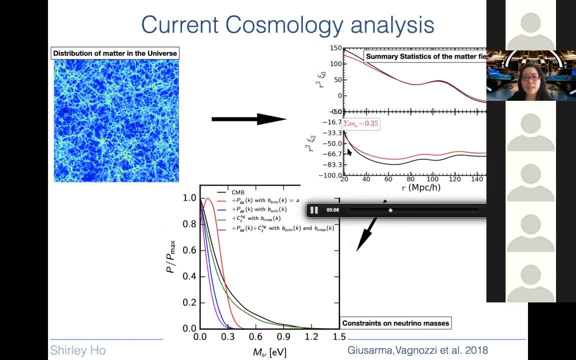 look at how you change some of neutrino masses and it changes the summary statistics also pretty dramatically when you hold all the other constants, basic cosmological parameters, constants- And you can take a look of what it is computed here from this map to this summary statistics. 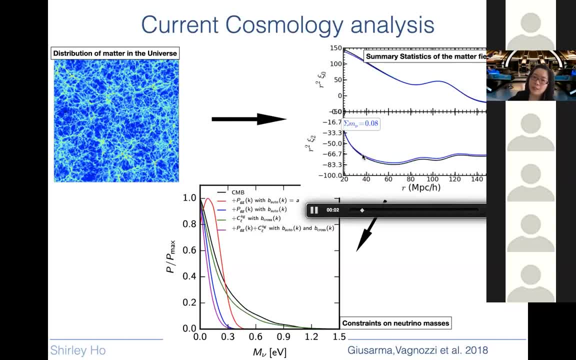 and compare to the theory, which is the predictions that we're just showing here, with this matching sum of neutrino masses And you can get a fairly good constraint on neutrino masses by combining CNB with larger structure, assuming different types of biases, either in 3D power spectrum. 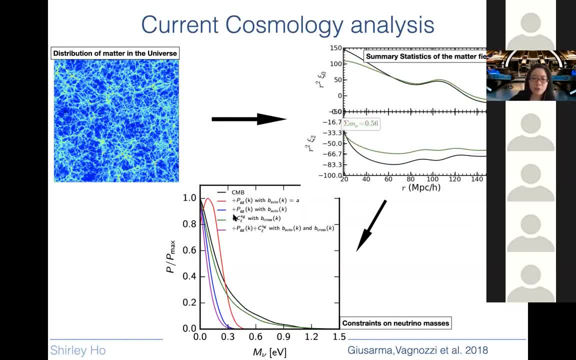 or the 2D power spectrum all combined, And how do you combine it with the cross correlation And that gives you a better constraint on neutrino masses. So these things are what I usually do and did I still do, actually sort of bread and butter. how cosmological analysis are done. 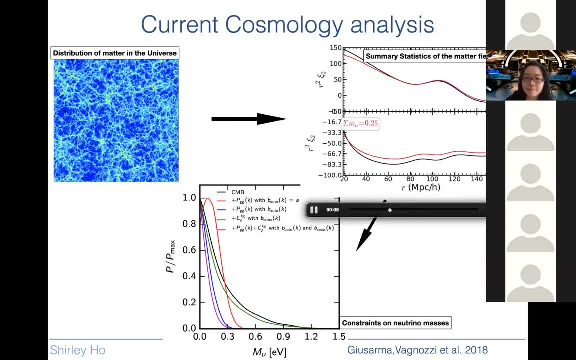 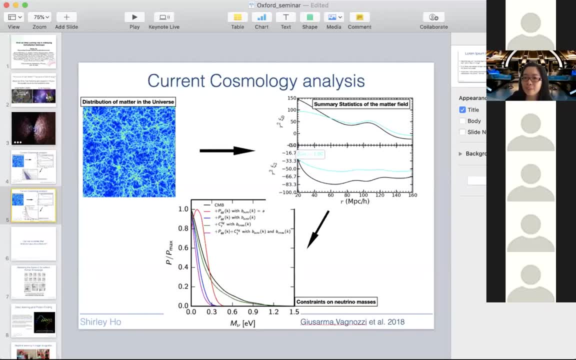 Is there any questions? first, Let me just pause. Let me pause for questions. So I just ran through, basically, cosmology analysis 101.. Yes, So there's the constraints. The constraint that I've heard on the sum of the neutrino masses is from cosmological data. 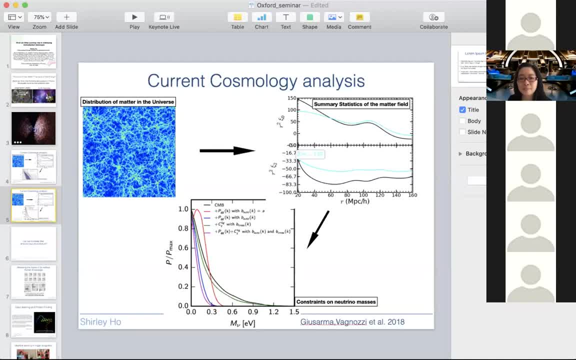 is 0.12 electron volts. Is that one of these combinations? There is many different combinations, but yes, this is. I think 0.12 is pretty low. I think it depends on which basically confidence intervals you're quoting. So is it two sigma, one sigma, or is it just a preliminary 95%? 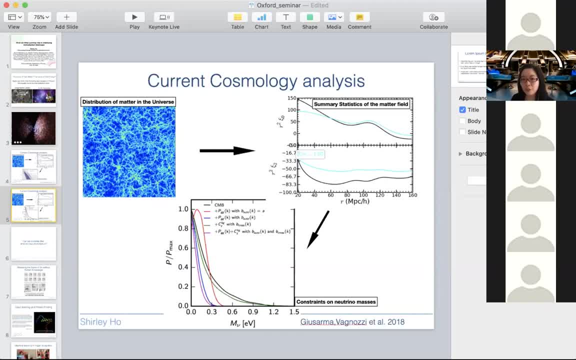 So yes. So when you say cosmology constraints on neutrinos, that's basically one of these combinations. Okay, Usually larger structure plus CMB. These are the two most. I guess people tend to trust it the most because they are all linear physics driven. 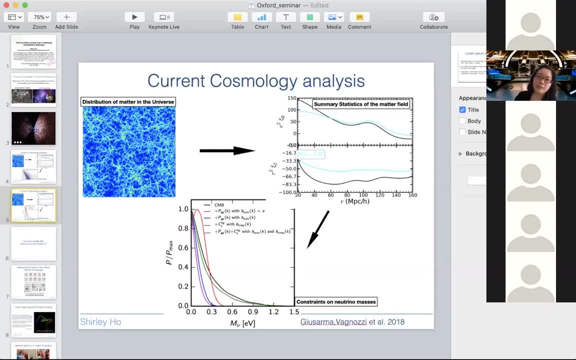 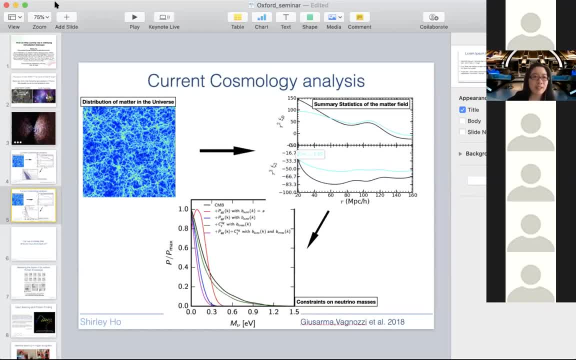 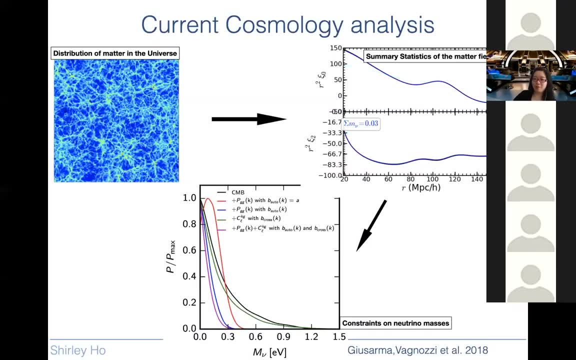 I personally found Zoom talks very difficult because I cannot judge if people are just falling asleep or already brewing the coffee to survive the talk. But we'll try. Feel free to ask questions. This is the easy part. So I was asking myself: can I do better than what we've done before? 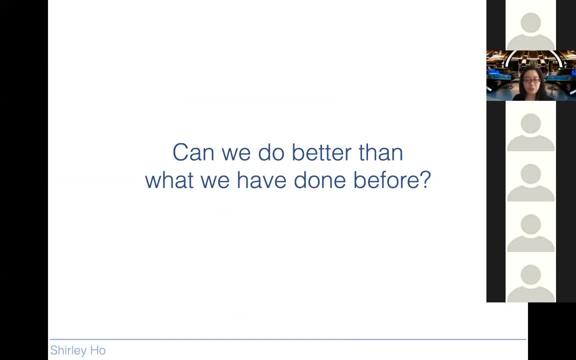 As all professors who got tenure tends to do, once you get tenure you decide you should do something different. Some people go off and want to become deans. some people go off and do something else. I decided to try something sort of different from what I usually do. 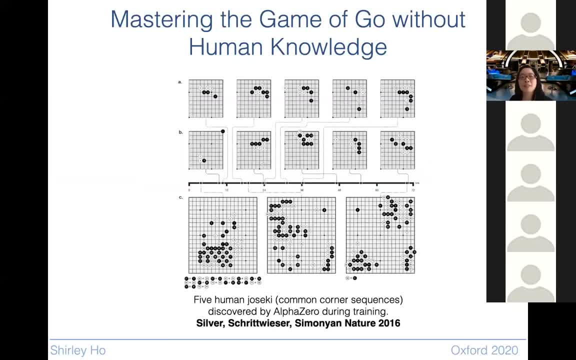 Because at that point there's a lot of, I guess, hype in machine learning And at some point you ask yourself: is there actual potential of really using it to transform in our field too? And it's also partially because I was in the field. 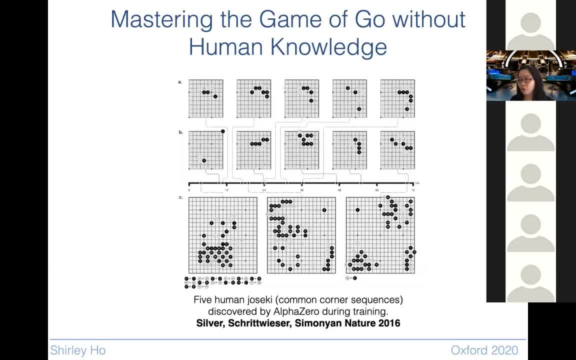 I was in Carnegie Mellon, which is very, very strong machine learning. I think it's the only place in the country that has a machine learning department of its own. it's their own hiring track and a computer science school of over 300 faculties. 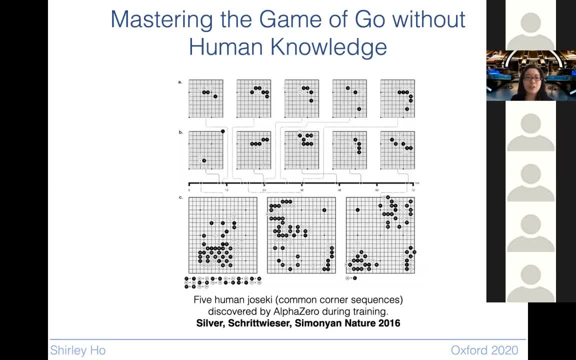 tenure track faculties. So everyone's talking about it, So I just decided to learn about it a little bit. And here's one of those things that you realize that they win against the best goal player in the world without you know even playing against these people. 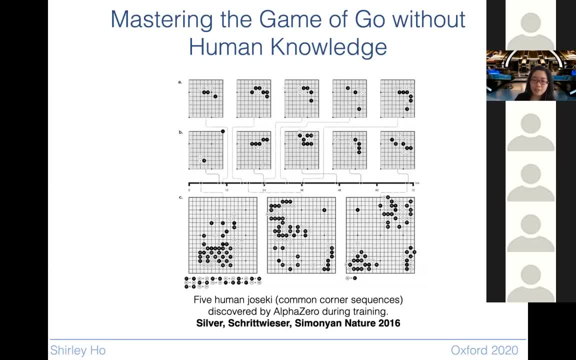 They train the machine, They play against itself And it is discovered the five human joseki, which are basically common corner sequences that are discovered during training, and even beats the gold champion in the world over many, many games, not just one game. 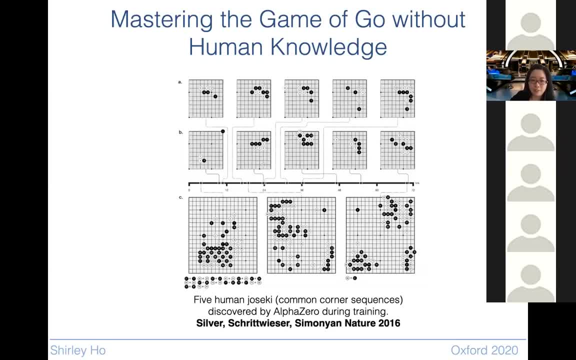 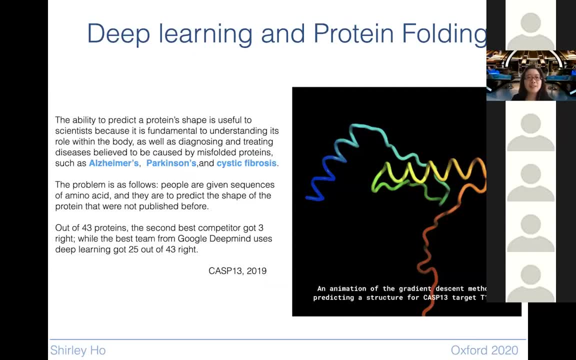 So that was pretty impressive. when the machine can beat, you know a human who's really good at playing goal in that game, And of course they've done a lot of other games since then- And then you're also something a bit more science driven right. 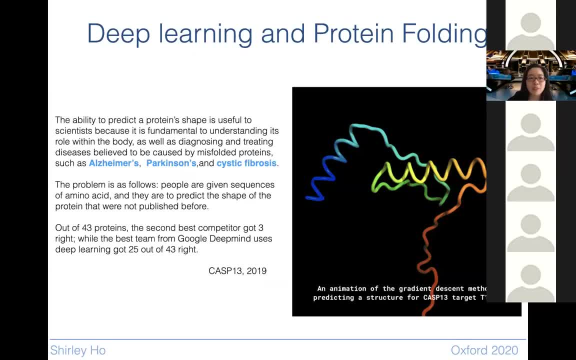 Because deep learning. So that's going to be very interesting. And actually I'm going to talk about something interesting that now I'm really interested in, which is the use of protein in protein folding. So protein folding- this is a very common issue in protein folding. 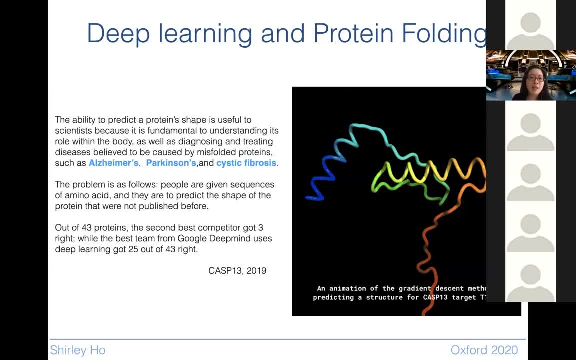 So it's something that is being discussed now in research And it's also applied to protein folding They recently had. So for people don't know about protein folding, it is very important because the ability to predict a protein shape. it's useful to the scientists because it's fundamental to understand. 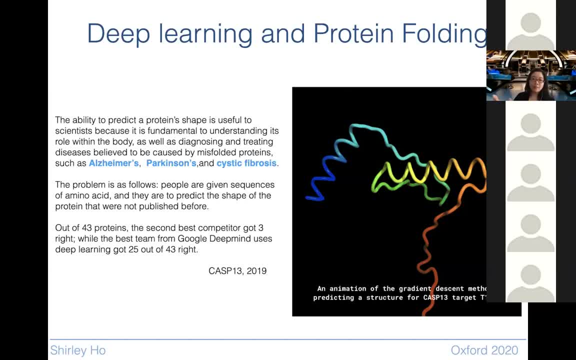 what it's doing in the body and they had to predict the shape of the protein that were not published before at all. So, out of 43 proteins, the second best competitor got three right, while the best team from Google DeepMind used this deep learning and got 25 out of 43 right. 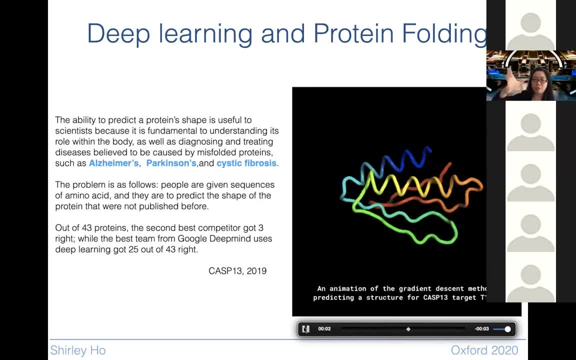 And here's an animation of what the gradient descent did you know so unfolded, and figure out how it's folded and predicted a structure for this target that no one has seen before. So I thought that was pretty cool. It even does something useful, not just playing games. 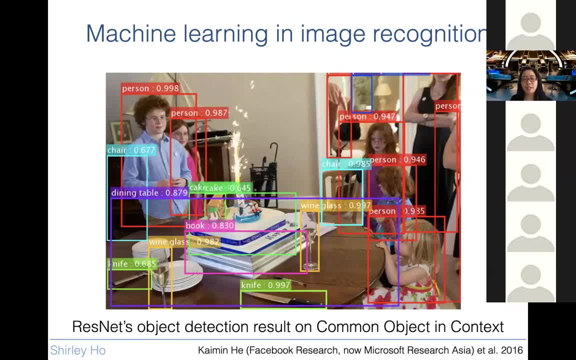 And something more commonly used is how to detect objects and figuring out what that object is, And this is using residual neural net, which also won the competition in 2016.. Things have changed a lot, but residual neural net is still used very heavily. 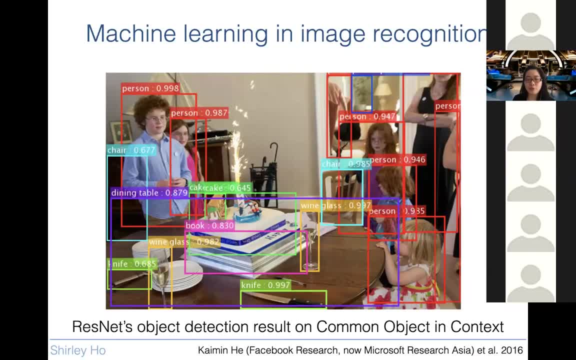 in image recognition since it performs so well And it won this common object in context competition, where you can see from here that the person was recognized very easily, even though they didn't have the data. Even a knife on the table or the wine glass is recognized in the cake too. 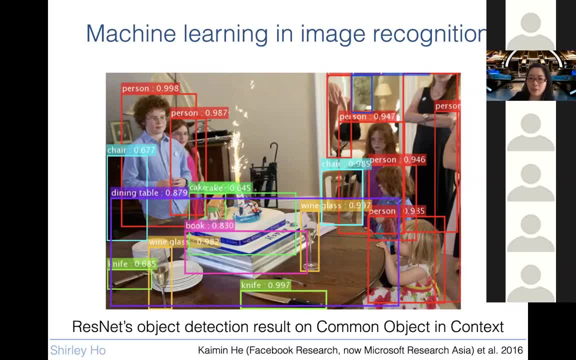 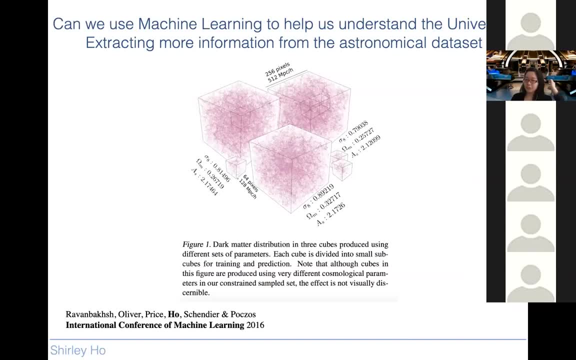 So with a probability which I think is quite interesting. So talking to people at CMU at that point. so Simon Rappenbach started early with us. He was actually a postdoc at that point with us, Me and Jeff Schneider and Barnabas Possos. 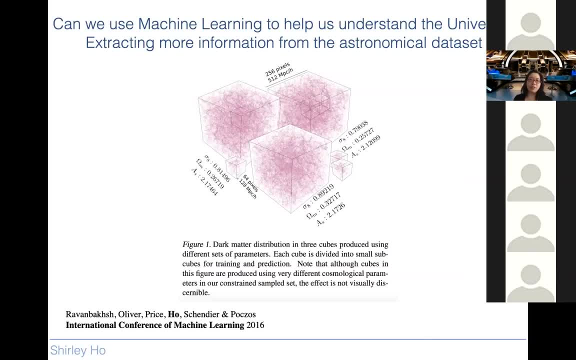 we looked at whether we can use machine learning as very simple project. You throw these cubes of different cosmological concepts, constants, So these large number of cubes have different cosmological parameters. By eyes you can barely tell the difference, because if you look at them, 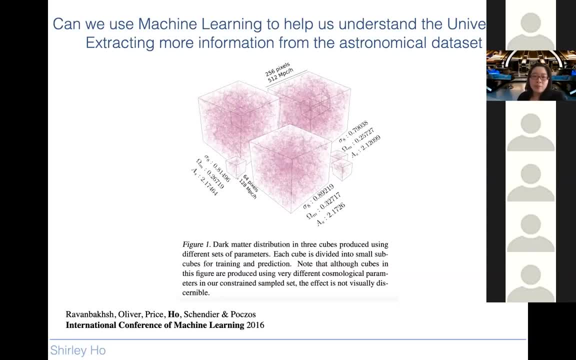 they basically look the same- The big ones and the small ones- shows you basically what we feed into the machine learning code, because at that point, this is 2016,. we remind you guys, there weren't even 3D convolution. It was the first paper we wrote, 3D convolution together. 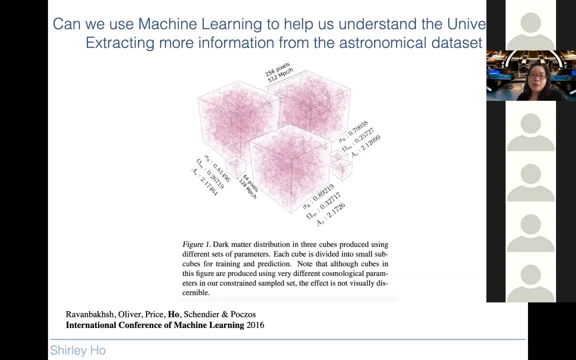 to do this work. There were also 2D and there isn't enough memory basically to feed the whole volume and you can only feed a tiny volume in. So we throw these things in and see whether we can extract more information from these data sets than what we traditionally do with. 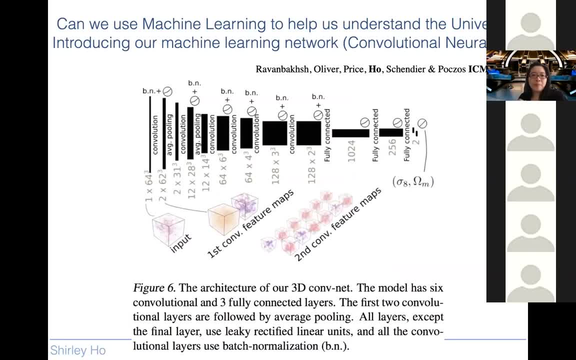 you remember all this correlation function we talked about earlier. So we throw this in on the left-hand side is the input, the right-hand side is the output, and you can see on the input these little cubes, the 64 cube, and you basically have a very simple neural net. 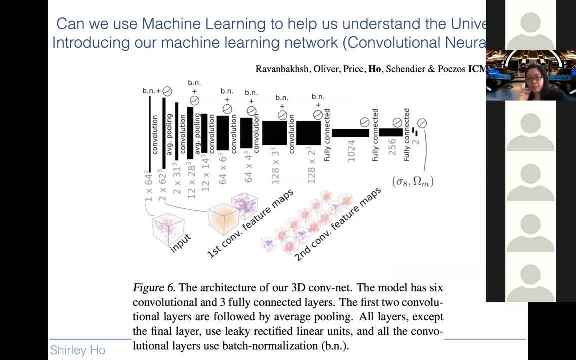 I mean now looking back in 2016,. things have changed dramatically. This is probably one of the simplest network you will start with right now. You have few layers and a six convolution: three fully connected layers. The details are not important. 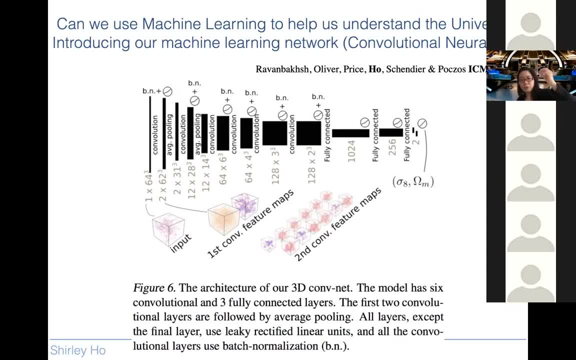 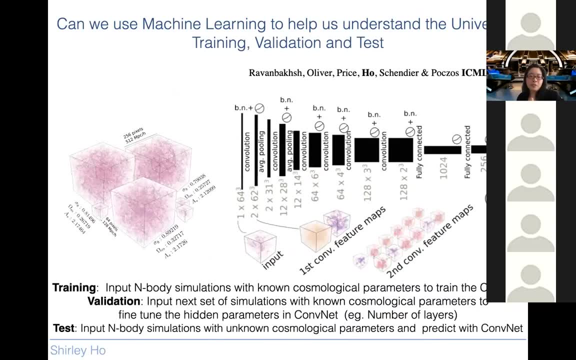 but what's important is that on the left-hand side you input cosmological cubes. on the right-hand side outputs cosmological parameter. So how does it do that? So you do it in three different steps. You have the input of the M-body simulations. 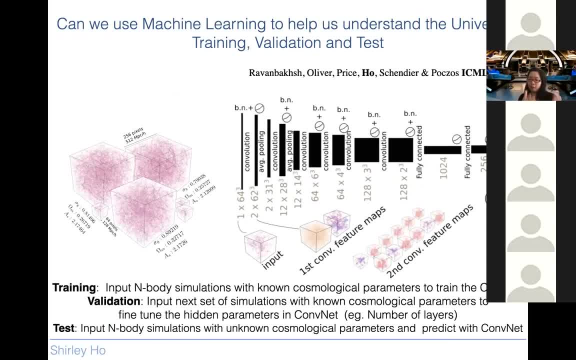 with known cosmological parameters. So you know what the cosmological parameters are. You have all the cubes. you train the network. When you train the network, you make the network learn all the different weights and constants and biases. There's a bunch of names. 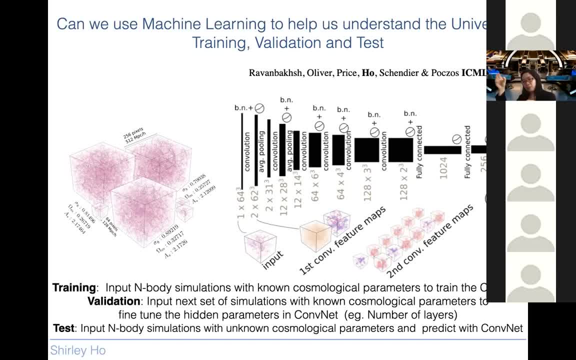 but basically it's tuning a network, tweaking all the knobs until it gives you the best results for omega matter and sigma eight, That they will match for all the cubes that you input, that you know what the output is, And then you input the next set of simulation for validating. 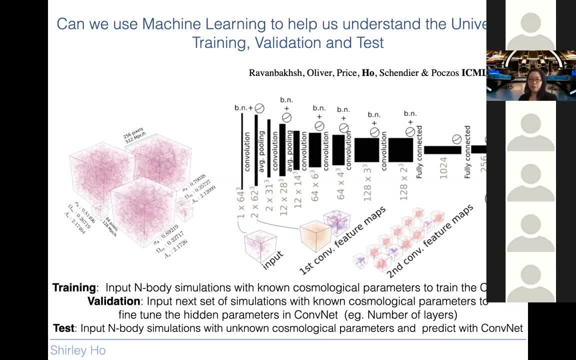 which basically usually means you want to fine tune all the hidden parameters of this neural net And test. that is what you do when you input M-body simulations with unknown cosmological parameters that you've never seen before. Well, the network has never seen before. 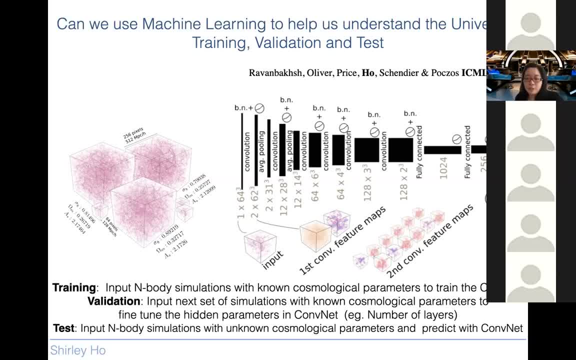 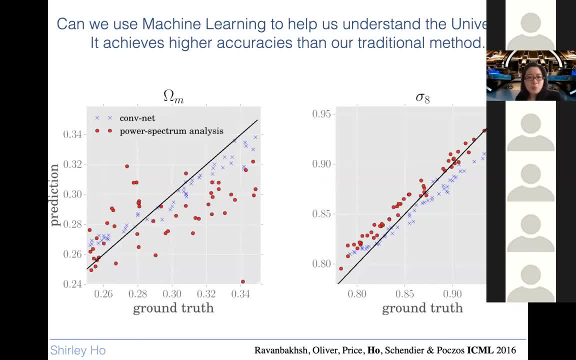 and see what the prediction went. This was published in the New York Times. This was published in the New York Times. This was published in the International Conference in Machine Learning, 2016.. And it's a long time ago. Here is what we showed. 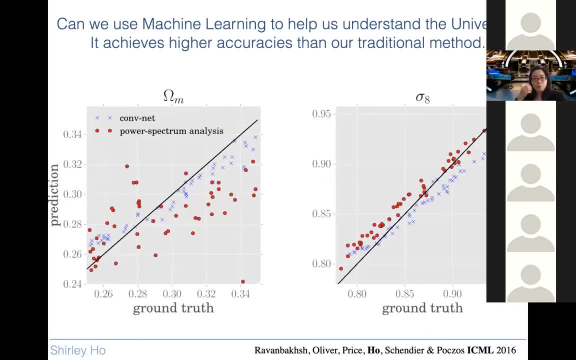 It's sort of upshot plot, You see, that the power spectrum analysis, which is what we usually do, has this huge spread. And it's not surprising for the cosmologists, because we only put in a very tiny cube. It's not the full cosmological volume that usually put in. 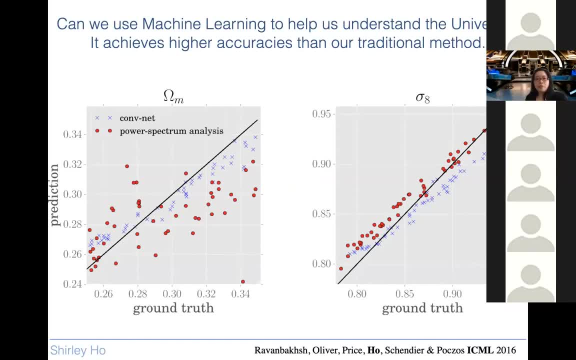 It's such a tiny cube you have a huge variance, While if you use the convolutional neural net you see this slightly biased. it definitely shrinkage of errors on omega matter. For sigma eight it's not as obvious, but it's definitely lines better than the red line. 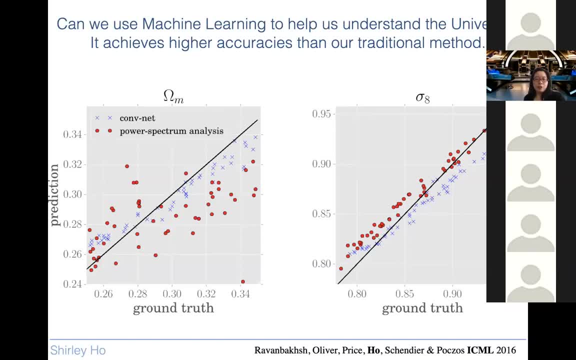 And later on we did actually redo this work and realizing that, retraining the network slightly better and tuning the network slightly better, it will achieve even less bias from the convolutional neural net. So, upshot, it does achieve high accuracy than our traditional methods. 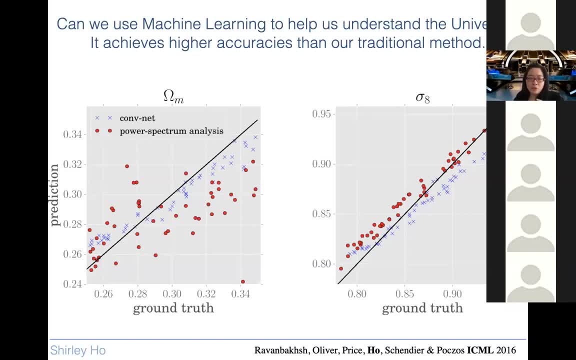 So I asked myself: whoa? okay, this is surprising. It was done in two months And we just want to try if it's going to do something better than what we usually do with my bread and butter analysis tools that sitting there. we've done it with Sloan. 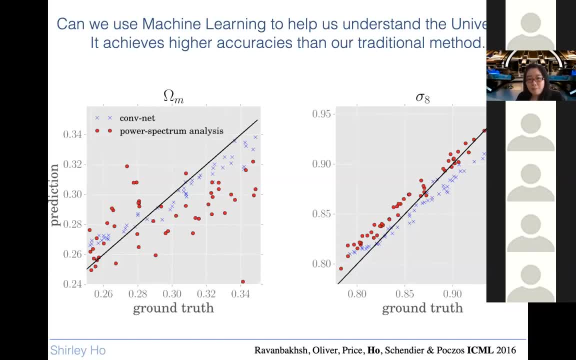 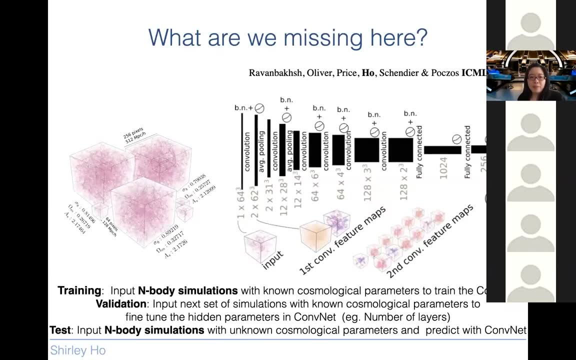 we've done it with BOSS So I figure it cannot be so bad, but it's not doing as well as the neural net. So what are we missing here? Let me just pause. if people have any questions, I would people you need to yell. 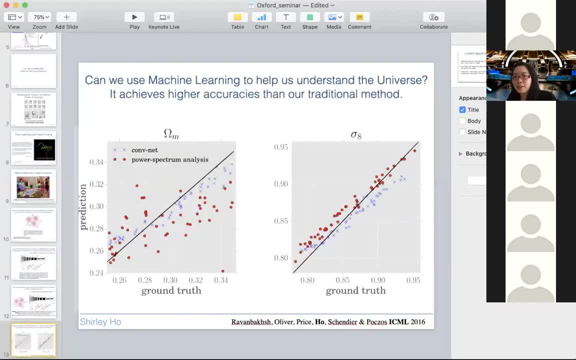 because I need to be able to see you talking. So how many different universes do you have to feed it to so that when you train it it can sort of tell you with another universe what the three interesting astrophysical parameters are? 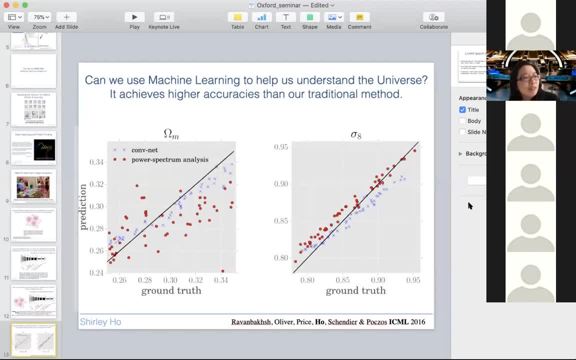 Yeah, so we used about I think 500 at that point, But honestly we did the whole analysis with slightly better tuned network. it's like a hundred And also depends on the volume of the universe and how complex your universe simulation is. 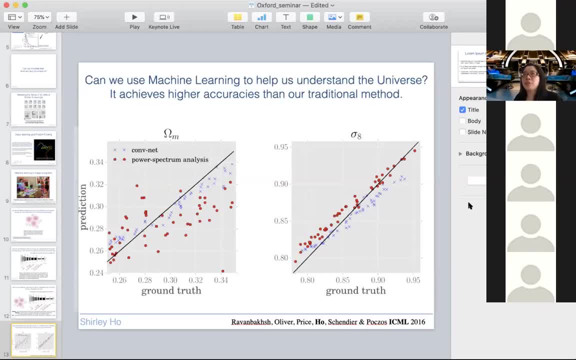 So when we use these simulations, they were not the most sophisticated and body simulations They were basically color simulations for people who are expressing cosmological simulations. They are not full, and body simulations They are basically fast, approximate simulations. So have less. how was that? I say? 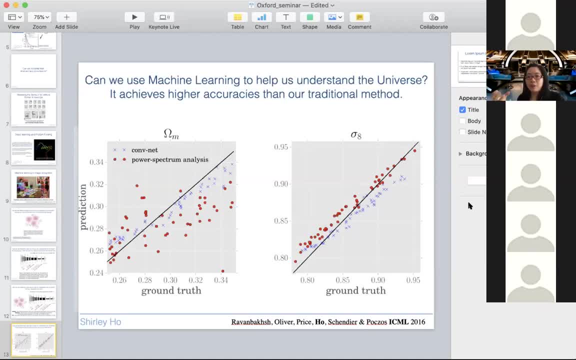 I would say that they're less information in each of these boxes. Well, when we switched recently to redo this analysis just for fun, for training for the students, if you take the true and body simulations like keyhole test simulations, 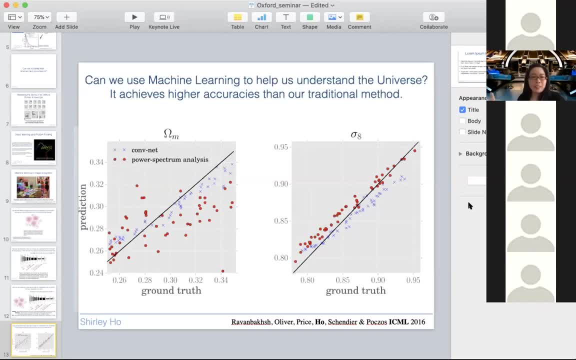 that Flatiron and Princeton has made it public. We have a petabytes of simulations. with how many? Over 20,000 simulations each one. get the parsec on the side And it was like really good, and by simulations We only took 10.. 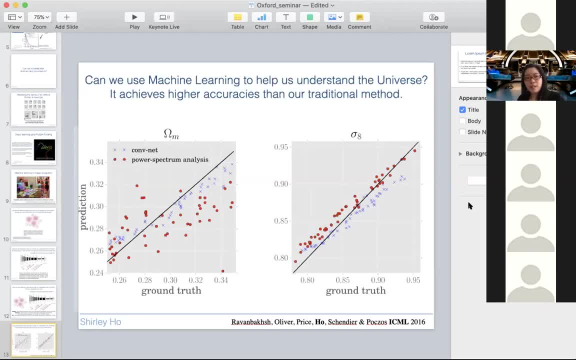 So that number, it's really really good, But that number is really not as important as basically how rich that data set is, I think at some level. But that's a good question. Anyone else has another question: Do you know what features the? 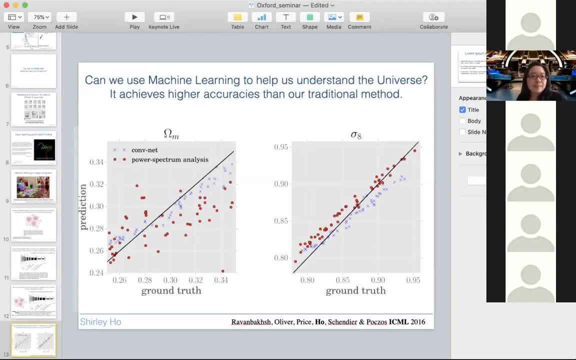 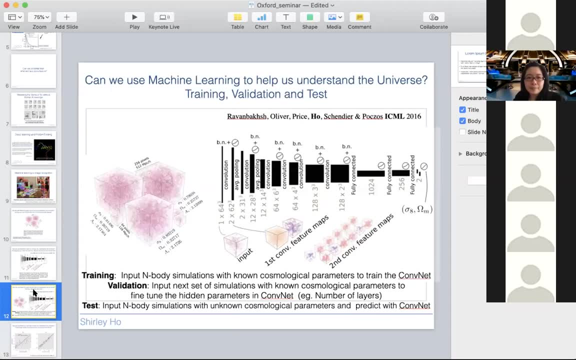 I mean you might be about to mention this- What sort of features, particularly in the Omega-M? what sort of features do you think that the convolutional, the neural net, is managing to get, that the regular sort of standard method isn't? 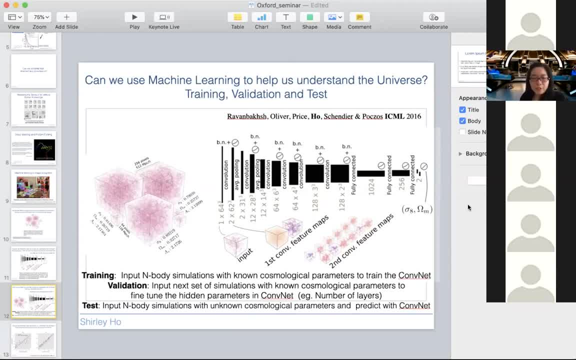 So we did not go too deep into it. As I mentioned, it was a work of two months, but we did look into this a little bit more in later different work. But for that paper we looked at different feature maps And I don't know if you can see my screen right now. 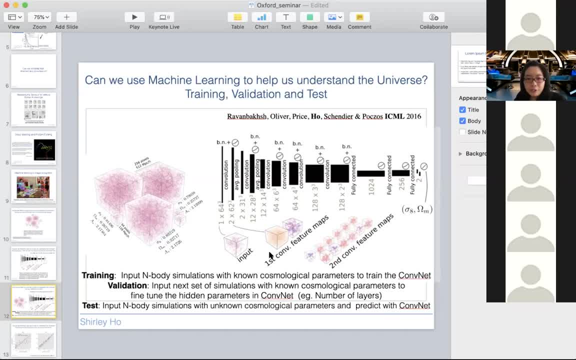 I hope you can. That's the first layer convolution feature map And the second layer convolution feature maps like basic second convolution layer And we pulled out the feature and see and try to look and see if there's anything obvious. So far nothing too obvious yet. 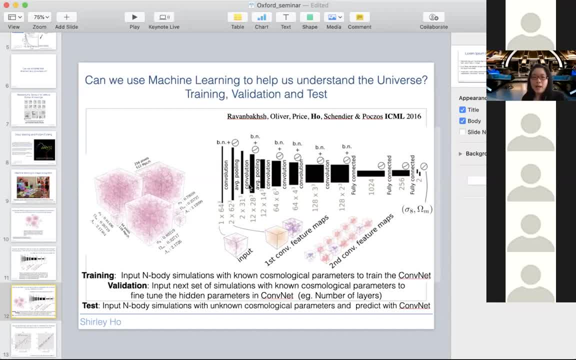 But you see structure. basically We had another work going on with the students. where we take, that's not publisher but we're writing it. where we take the cosmological simulation boxes, we put it into an autoencoder which basically 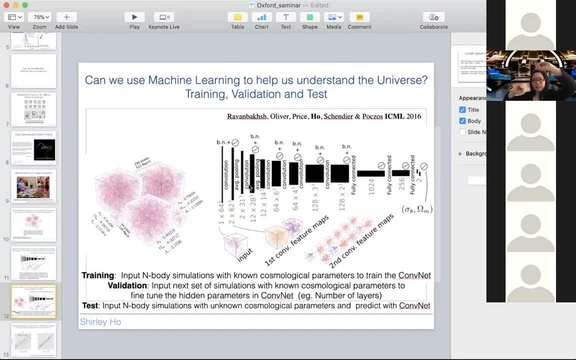 so do multiple convolution, compressing the data basically, and then try to look at in that bottleneck where things are compressed with least amount of bytes, basically contain that information And then look at for each of them how it correlates with different cosmological parameters. 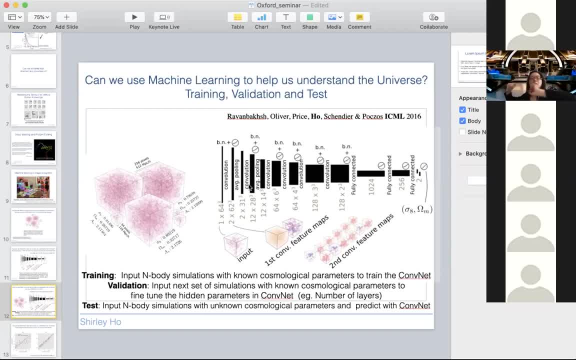 and what it looks like If you take each factor, what it looks like And it's interesting. it's not obvious what they are, but some of them do have do kind of look like. I don't know if people looked at wavelets, for example. 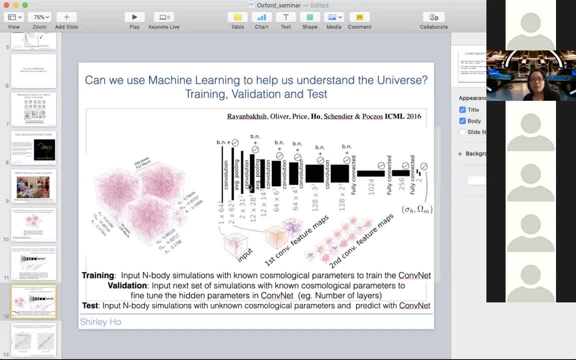 It has some similar features of wavelets. It's not what you expect with clusters and filaments, but it's more like wavelet where you have for different scales, they have different directions of filamentary structure. So that's what we saw so far. 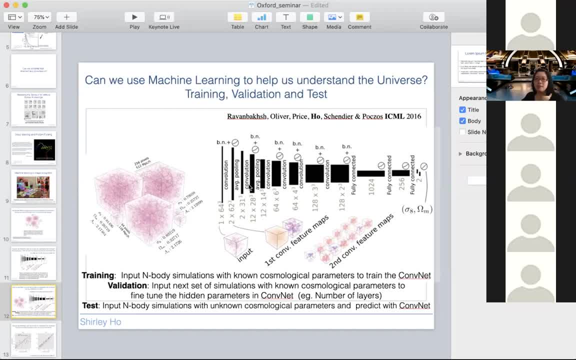 but there's a lot of work to be done there too, because- but that's another talk- if you wanna go there, But it's a really great question to look at the representation What basically Neuronet is learning here, And then you use the tuned network on the real universe. 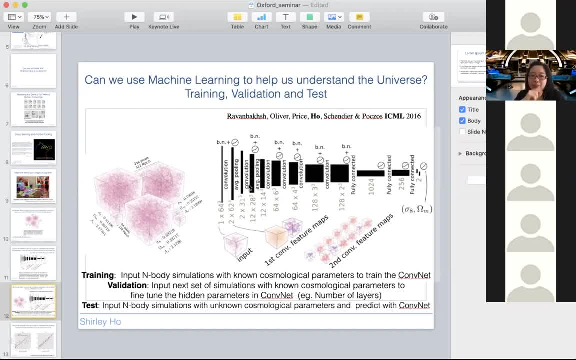 to extract parameters? Not yet, but that's the next part of the talk And I'll explain why we need to do a bit more work to use the real universe here, Because, if you notice, these are similar universes and they only embody simulation. 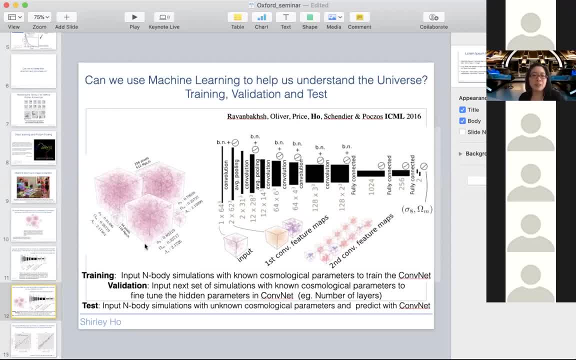 They're not even true embolism. They're fast, approximate and body simulations of dark matter only, And our universe is way more complex than that. And our universe is way more complex than that. And our universe is way more complex than that. 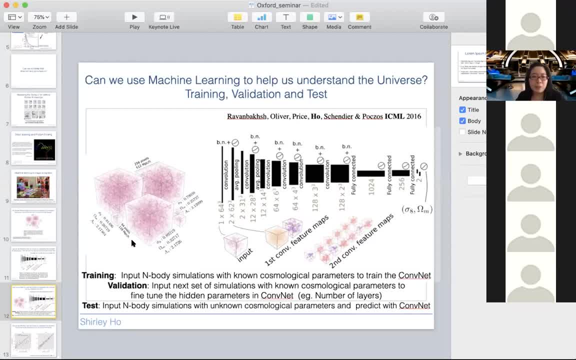 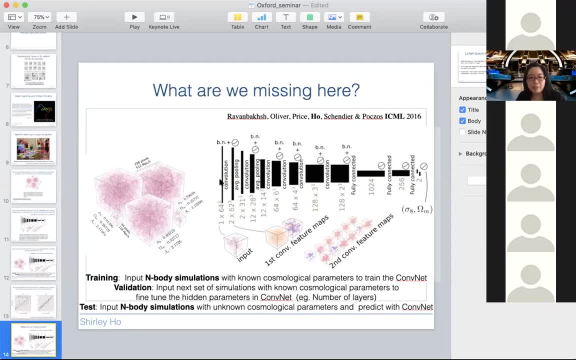 So you actually just preempted my introduction. What happened next is that? what are we missing here? right, We're inputting embolism simulations, basically of dark matter, to try to get the cosmological parameters, But what we really need is true: 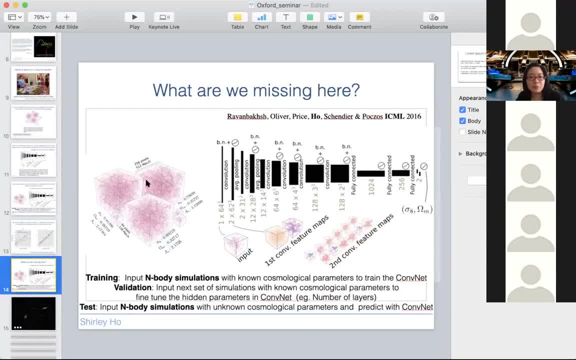 you know, looking like a universe that we actually observed. but I can go and continue that part of the talk. Any other questions before I move on to the next question? Any other questions before I move on to the next question? Any other questions before I move on to the next question? 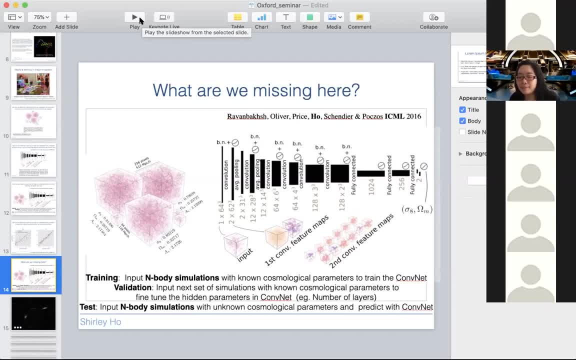 Any other questions before I move on to the next part of the talk, Because that will answer the last question, Because that will answer the last question, Because that will answer the last question, All right, So, as I was saying, now we're inputting these fake, not fake. 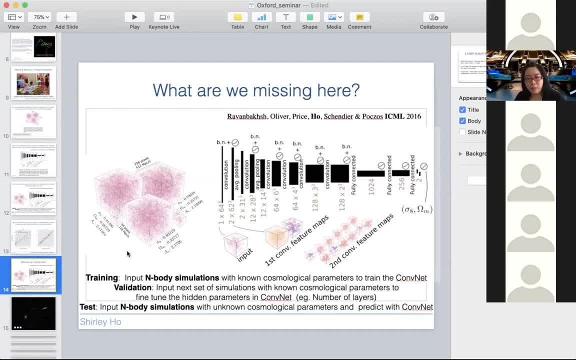 but basically simulated universes that are not very correctly representing our universe. So we want to actually input a true universe here and output the cosmological parameters. Or you can make comparisons, which people tend to do directly from the observed data sets to something that truly look like our universe, with all the 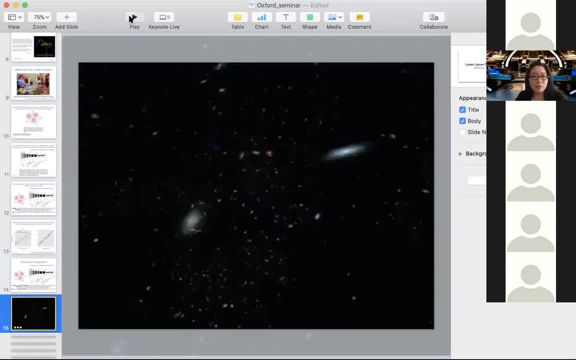 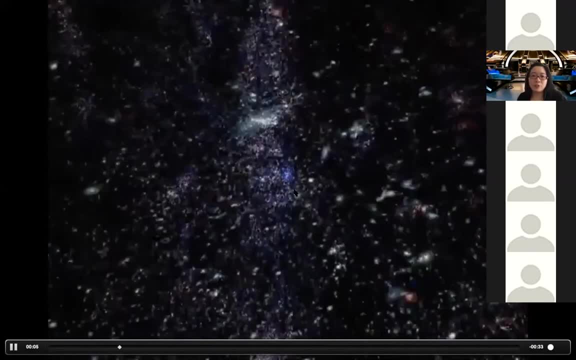 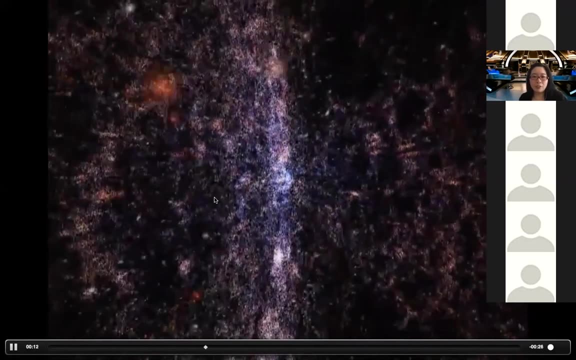 imperfection and the perfection. So we want a universe that looks sort of like this- right, Because right now we only have this- is Sloan Digital Sky Survey. what they actually see when you look into the sky. Every single galaxy is real image of the universe. That's why it's blobby. 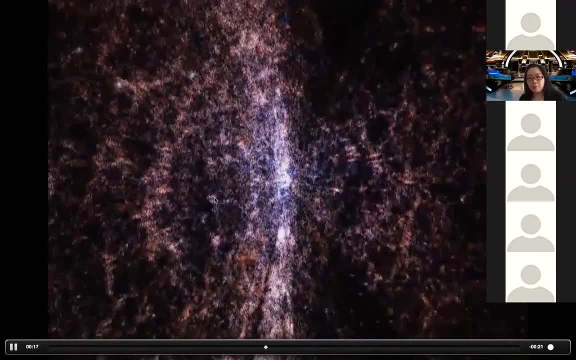 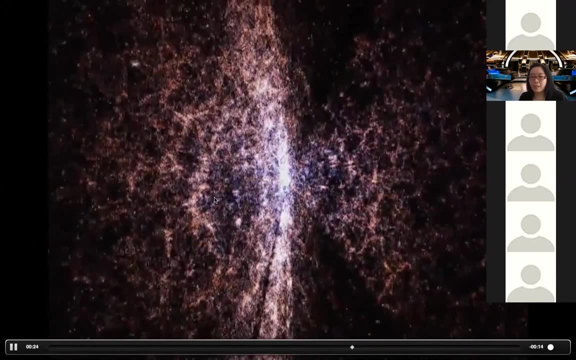 the further away you go, You're flying out from Earth. Basically, that's where the telescope looks like. look at and you can see this larger structure. We want something this complex because you want to compare your data that you observe, say if it's Sloan Telescope or Euclid. 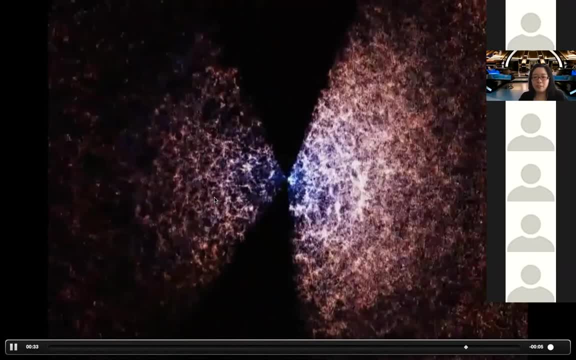 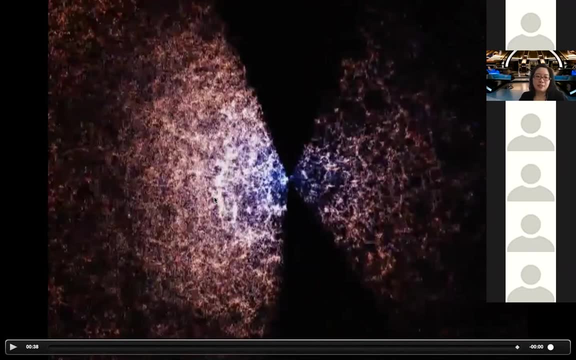 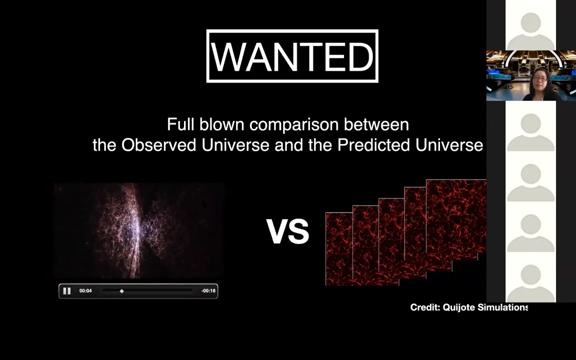 or you know, 2MASS, whatever you want to look at, or BOSS, and realizing that this is not so easy to simulate. So that's the next part of to talk Interesting, Okay. so what do we want? What we want here is full-blown comparison between the observed. 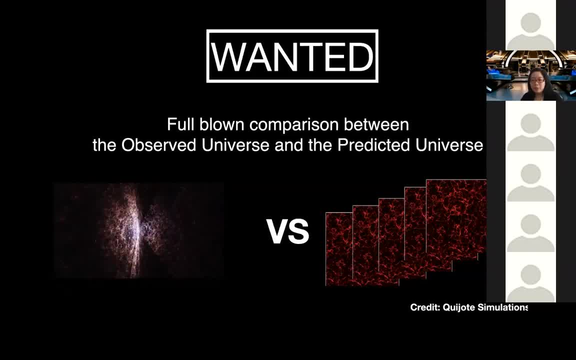 universe versus the predicted universe. So the predicted universe here, even though I use quixotic simulations, which is mostly dark matter. it's just the dark matter simulations, but we want the full-blown one, which means includes hydrodynamics. You need to know what the galaxies look like. 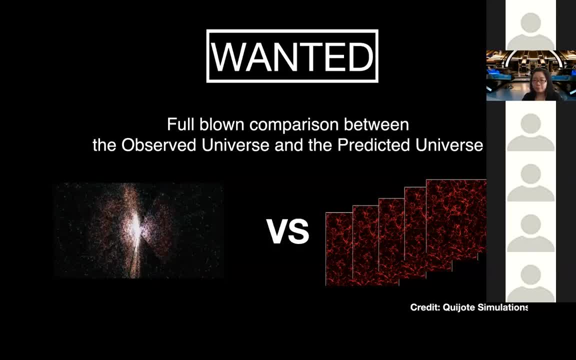 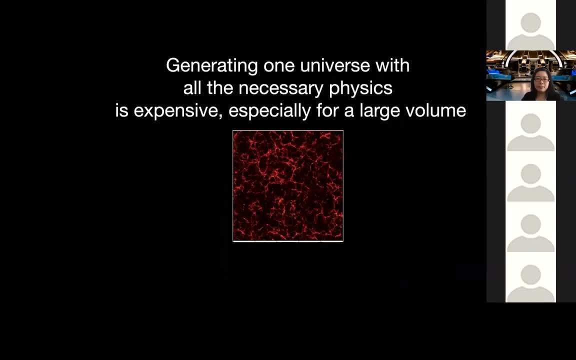 so that you can actually use this to train the network right Like something that's looking like the real universe, to train the network before it can input the true universe there. So generating one universe with all the necessary physics is expensive, and especially for large volume. For N-body dark matter only is not that expensive. 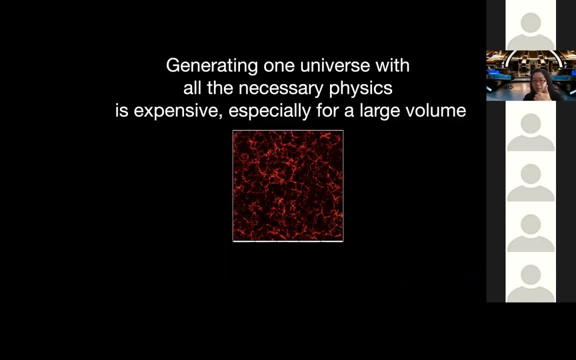 It's completely doable. but still, when you want many, many of them, it could be expensive. But with, say, one single gravity, only dark matter, simulation of reasonable chunk of the universe, say a gigaparsec on the side, takes about 1.8 million CPU seconds. So I'm using seconds for a reason you'll see soon. 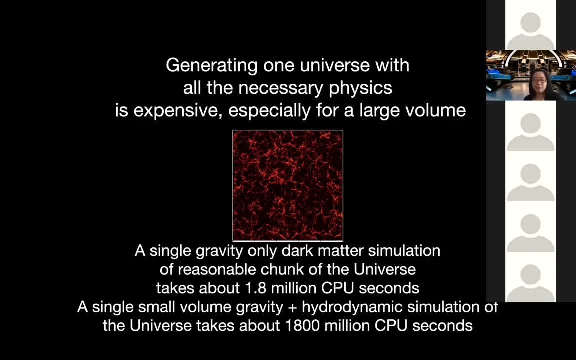 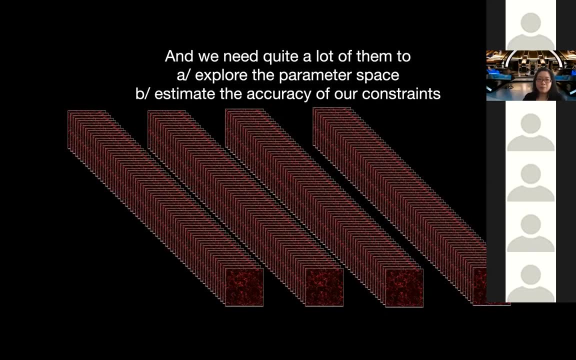 And a small single volume: gravity plus hydrodynamic simulations of the universe. that includes baryons, dark matter, you know, gas particles, all that stuff. the universe takes about 1800 or 1800 million CPU seconds. Those are some serious numbers And we need quite a lot of them. 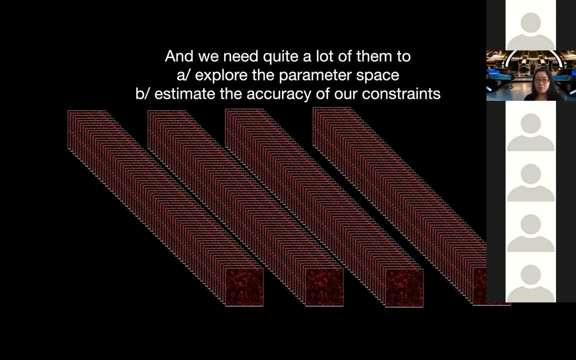 to explore: A- the cosmological parameter space. B- you want to estimate the accuracy of our constraints, And the parameter space in aid I mentioned here is not just cosmological parameters but also various astrophysical parameters. that connects from the dark matter evolution. 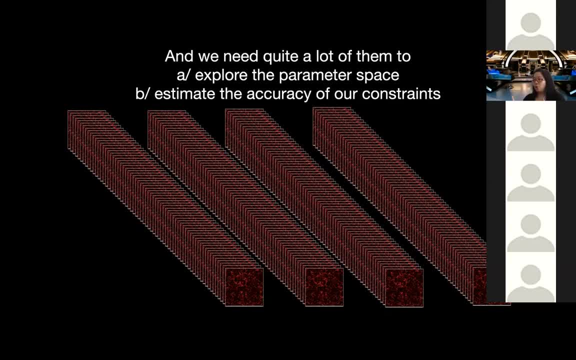 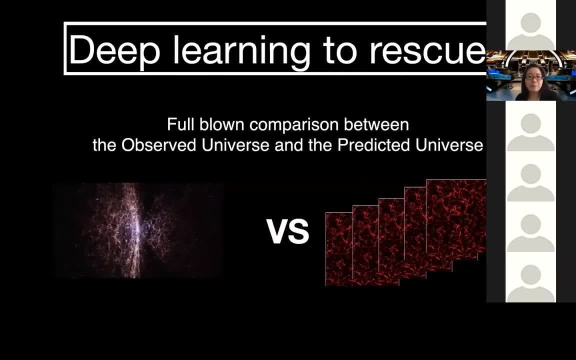 or basic underlying evolution to you know the galaxies itself, what the light will come out. you know what kind of light will come out. what would you observe? So can we do that? So I claim that deep learning is coming to a rescue here. 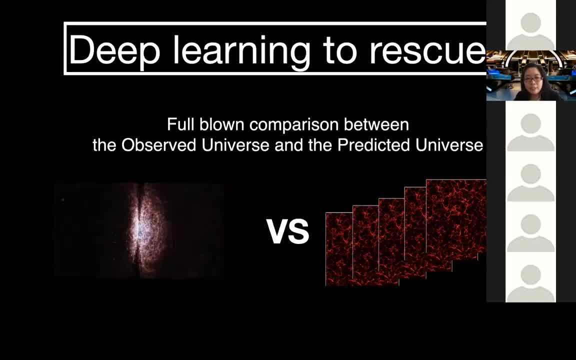 And we will try to do a full blown comparison. And this comparison you don't necessarily need to do with deep learning, which was what I suggested earlier, But you can also do it with traditional methods. People like to talk about like this: likelihood, free inference. 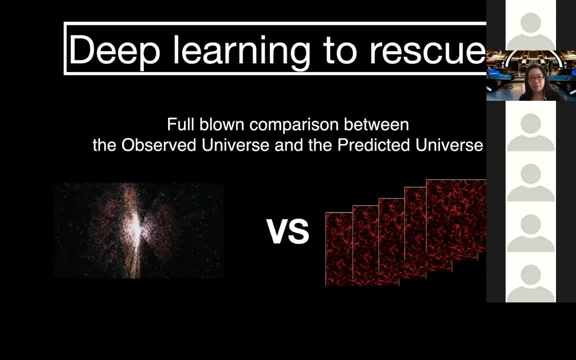 you can do however you want to compare- because the comparison is a different set of tools- that you can do. a near net. you can do, you know, full blown comparison with various different MCMC methods. You can also do reinforcement learning with current inference machines. 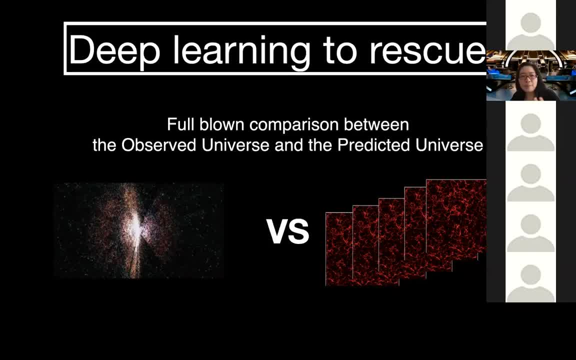 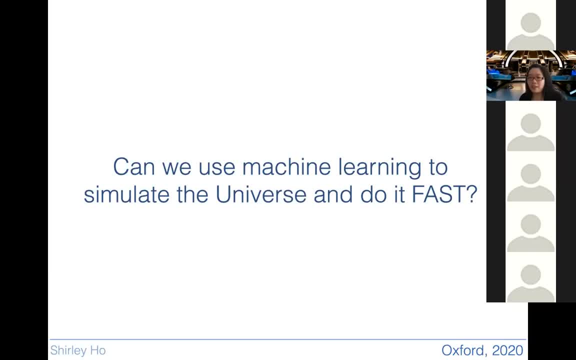 there are many possibilities, So I'm not going to go to that. But today I'm going to talk about how do we use the universe to simulate the universe. how do you use machine learning to simulate the universe and do it fast. So that's what I'm going to do today. 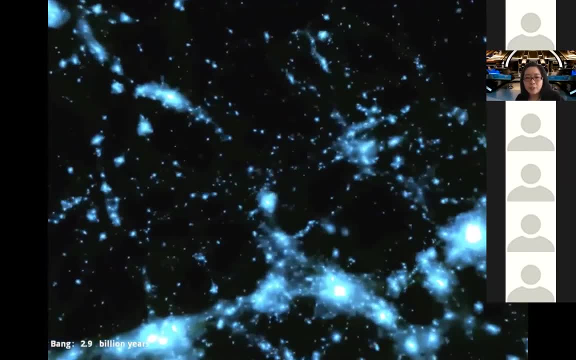 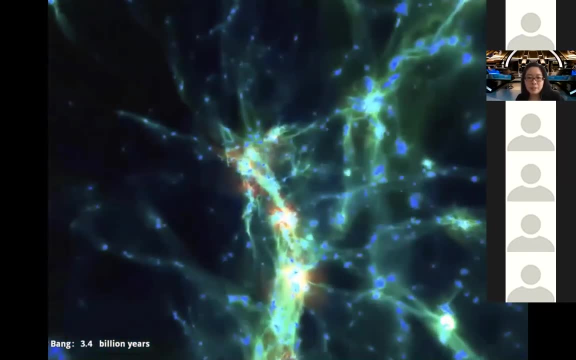 So here is a simulation that we actually want to, we actually using as a training set. that's what we want to simulate very fast. It is currently at 3.2 billion years and you probably will see some interesting explosion from supernova And this is showing. 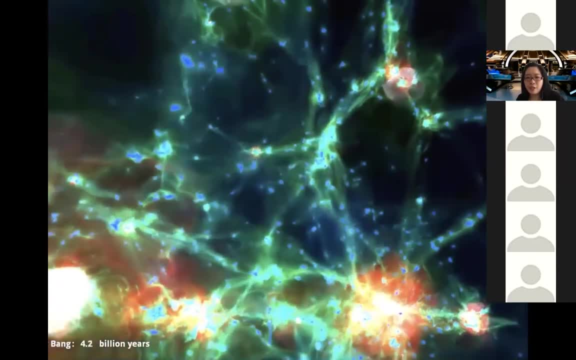 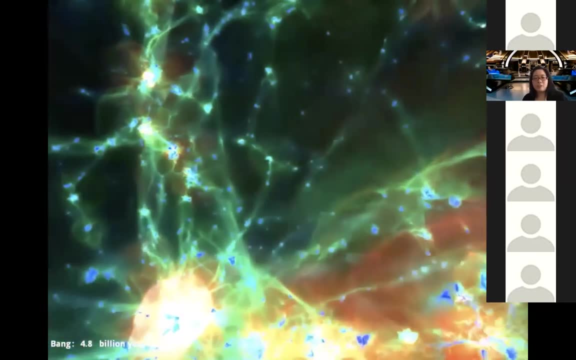 the temperature map of the universe And you can see this fairly complex things are happening everywhere. It does affect how massive the galaxies are. you know if there's stuff more blown out from the area, the more gas being blown out maybe changes the formation of the galaxies. 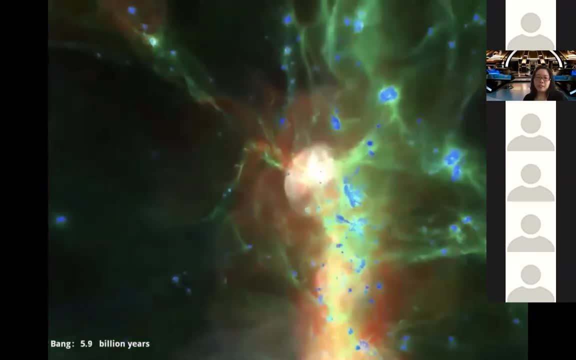 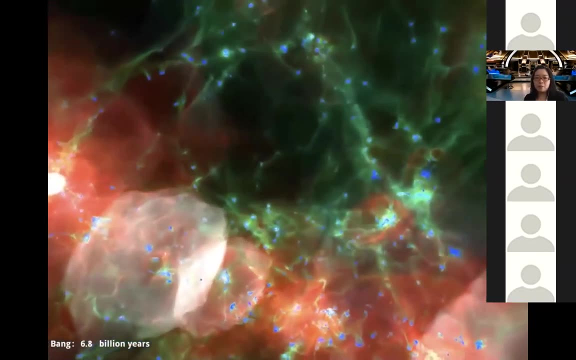 and changes to galaxy properties that we observe And, in turns, tell you something different About the universe, depending on how you model this and how you compare it with the observation. So it's pretty complex And I thought it's really beautiful at the same time. 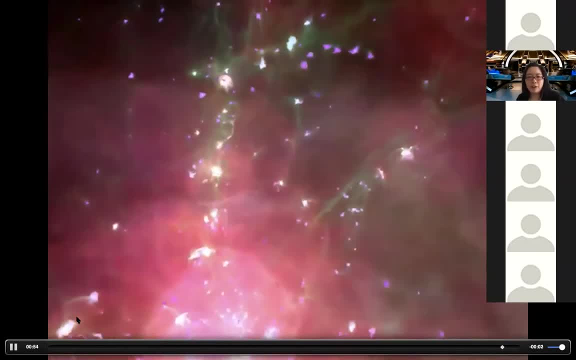 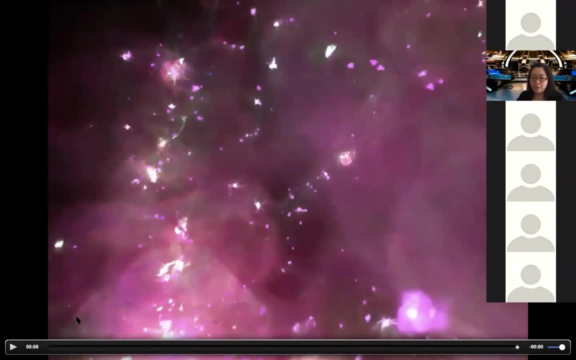 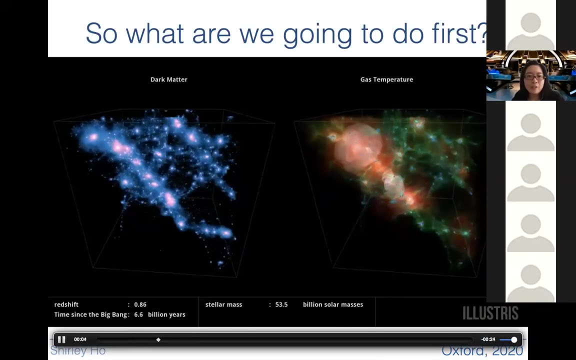 It's hydrodynamics, fully in there with gravity, And here I think it changes color- is the metals, So that, as for the physicists, here the metals is anything beyond like helium. So what we're going to do first, on the left hand side, we have the dark matter. 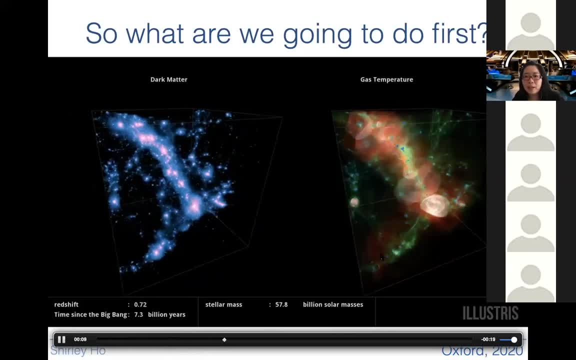 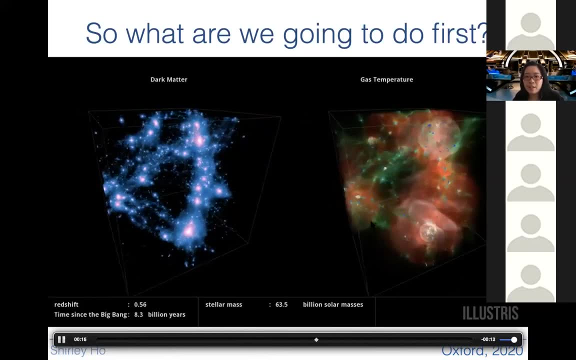 simulation, And what we're going to do next is we're going to do a very simple simulation that looks way simpler. While the gas temperature, you can see all the explosion of supernova causing very huge variety of variances in gas temperature, And he's just showing you. 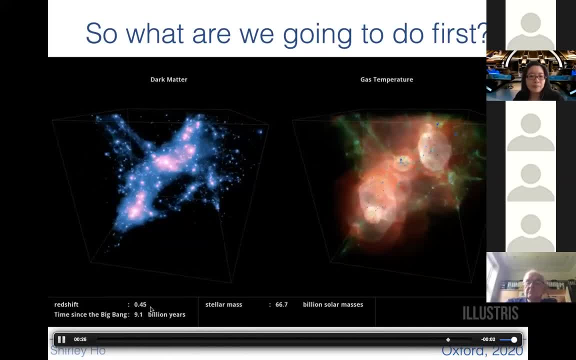 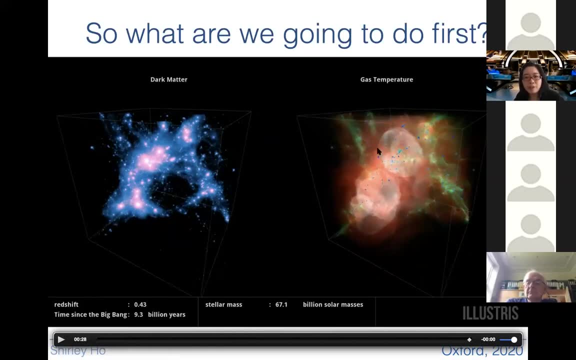 the different redshift as it goes down to 0.5, 0.49,. it keeps going down And you can see it's pretty complex, but all this time the gas temperature is so much bigger than the air temperature map. 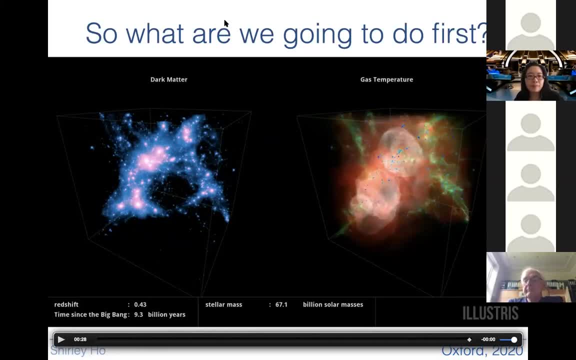 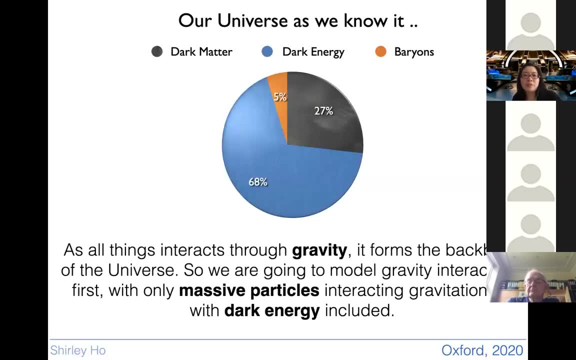 so it follows the dark matter map, which is very important. So the universe as we know it, we have the dark matter, the dark energy, with the variance, and all things interact with gravity. as I just showed earlier, it forms the backbone of the universe. 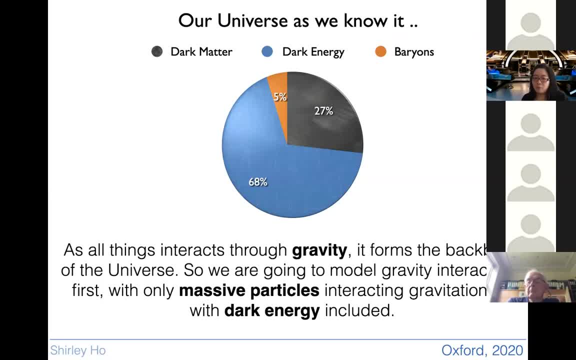 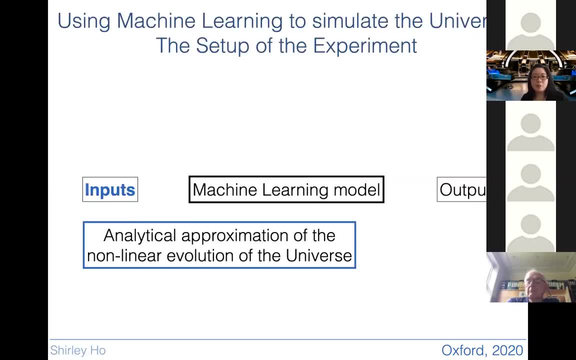 So we want to model the gravity interaction first, because it still takes 1.8 million Cp seconds to make one with only the massive particles interacting gravitationally with dark energy included. So what do we do here? We want to use machine learning to similar universe, but only the 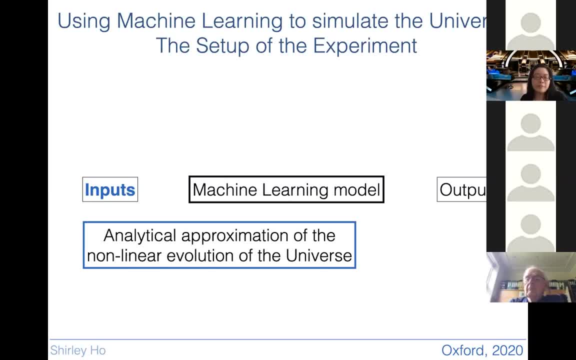 gravity side first, and we'll go to the next part later. The input is an analytical approximation of the nonlinear evolution of the universe. The output is positions and velocities of all the particles evolving the gravity after x years and we have machine learning model in the middle. 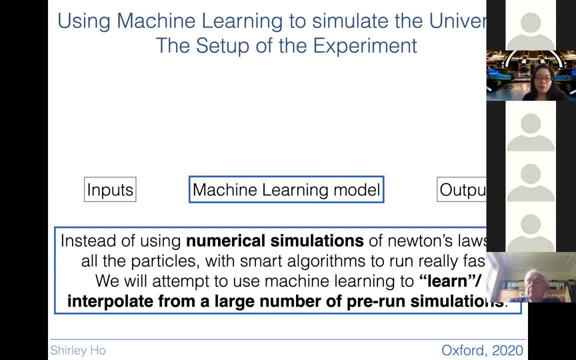 instead of the numerical simulations or Newton's law for all the particles with really good smart algorithms running really fast- and 1.8 million cpu seconds was not slow, given the scale of things- We attempt to use machine learning to learn or interpolate from a large number of pre-run. 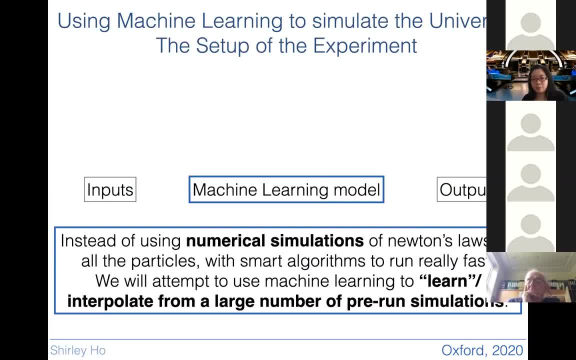 simulations and people actually ask me how many number of simulations I actually needed For the work that's published here. we use these fast pm simulations and we needed about a thousand, but recently we re-ran a bunch of this, this work, with this complex simulations that are full and body. we only took 10. 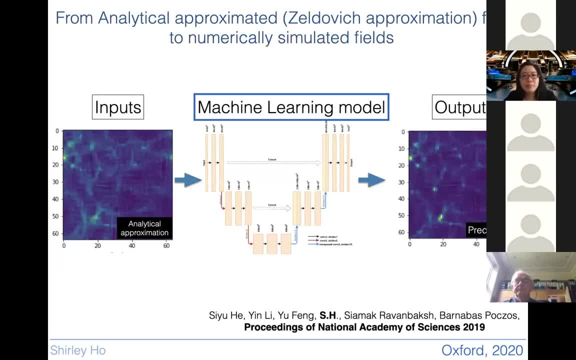 and it did equally well. So we go from analytical approximation, something called established approximation field, to numerical simulated field on the right. So on the left hand side is the input, on the right hand side is the output and something in the middle is this machine learning model that we used. this is work recently published, left by my students. who's 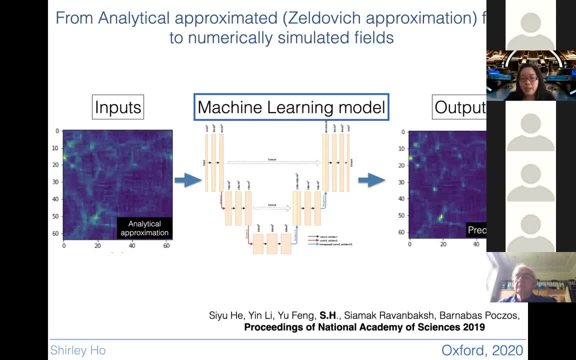 now graduated CUA. I'm going to show you how to do this. So I'm going to show you how to do this. I'm going to show you how to use network modelling as published in proceedings National Academy of Sciences in summer, and the network model is fairly simple: it's this residual neuronet. 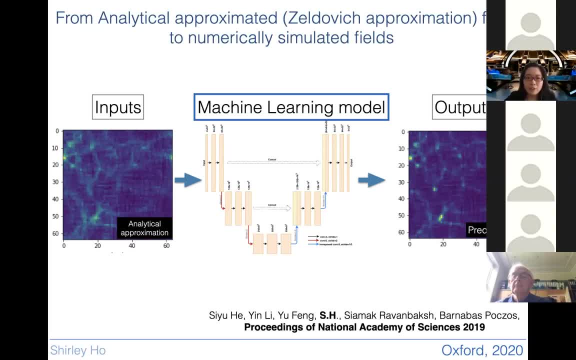 but in U shape. That's why people call it u-net. it has some interesting concatenation in the middle. that is required because you want to have the large-scale information coming in to the output. still, because the large-scale analytical approximation is still correct. It's the small scale that's wrong. 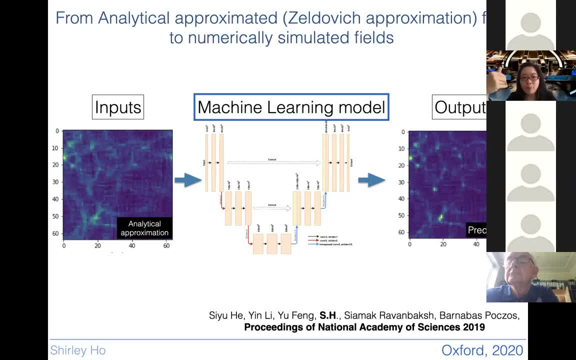 machine learning to learn what's needed but also take from the input what is good. so that's sort of some design of the architecture and thought went into it and then you see it dropping, going down. it's basically every single time. you can kind of think of it. they conform with different scales. 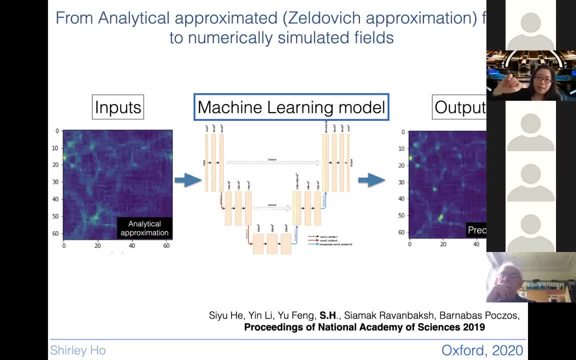 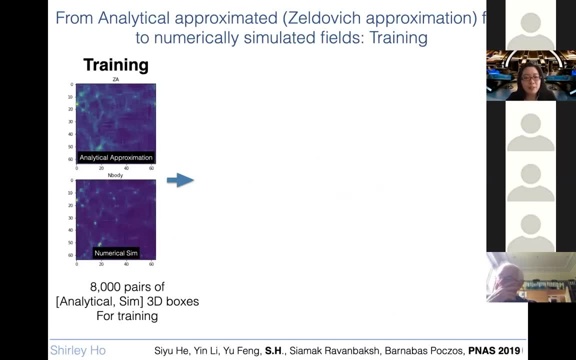 and collapsing the information into the bottom. it's called the bottleneck, and you can expand it back up into the predictions. so what do we do? actually 8 000 pairs of simulations boxes, but again we only need the 10. right now. we just realized when you use the complex simulations. 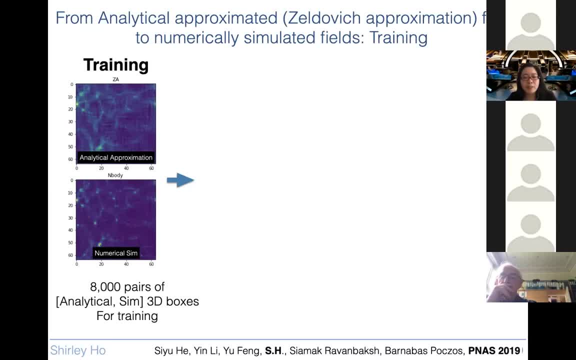 we have 8 000 pairs of 3d boxes for training and these pairs are analytical approximation on the top and numerical simulations in the bottom. you feed it to the neural nets, which is- uh, it's called unit. it's slight variance to residual neural net that people usually use. 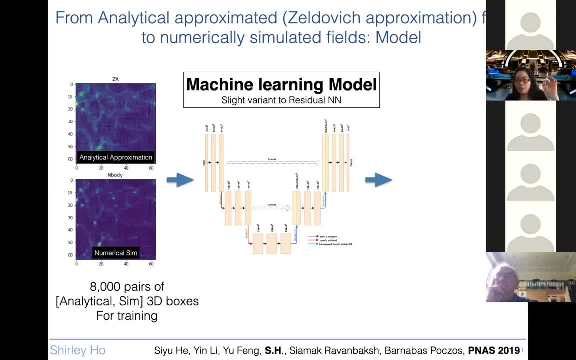 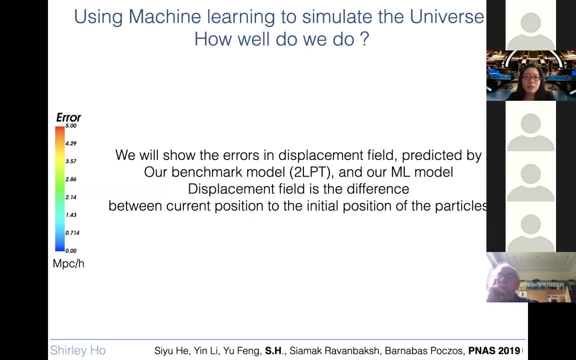 to do image recognitions- whether it's a person that i talked about earlier- and then input and output looks really good. soon i'll show you why. so let me show you how well we do. we first will show the errors in displacement field protected by a our benchmark model, which is 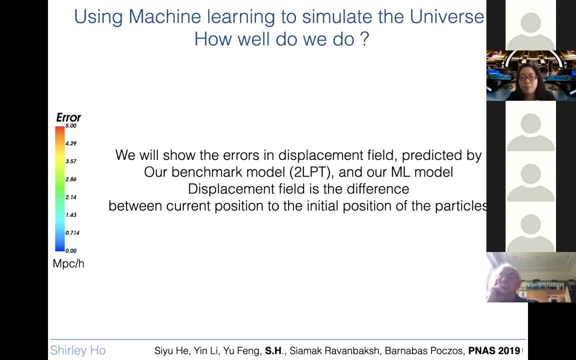 2lpt, which runs really fast. it's second level perturbation theory. in our machine learning model. the displacement field is just the difference between the current position and initial positions of the particles. so we're going to show you how it works and then we're going to show you how it works in the next. 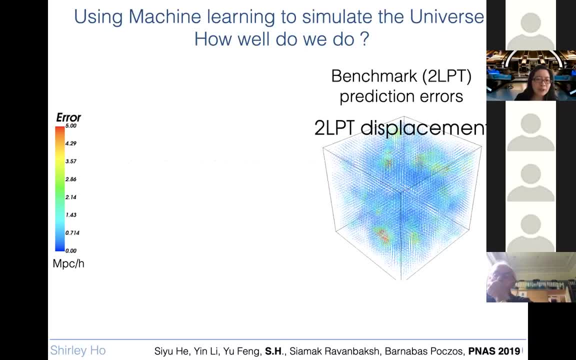 slide. so here's how our benchmark performed. it performed fine. i mean, the error bar here shown is mega part microposite over h, and the maximum error i ever got was five microposite over h, and most of the place is zero or to 0.7 and it actually strongly correlates with the overdense. 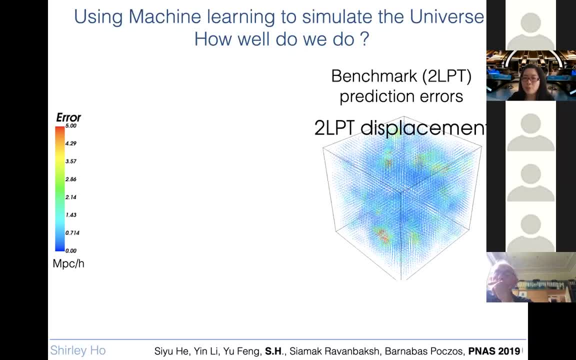 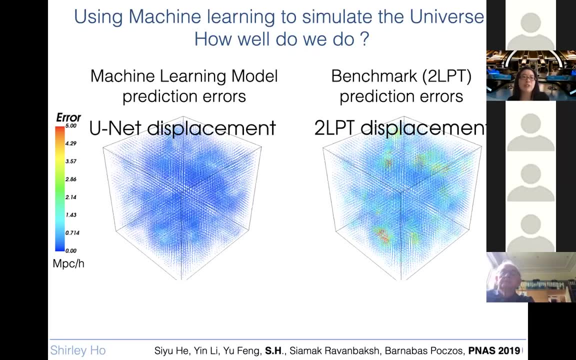 region. you see that when it's overdense it's less well modeled and i think we have some reasons to believe why that's the case. and for the machine learning model you can see that the unit displacement field it looks really good. it basically has no red and if you look at the numerical 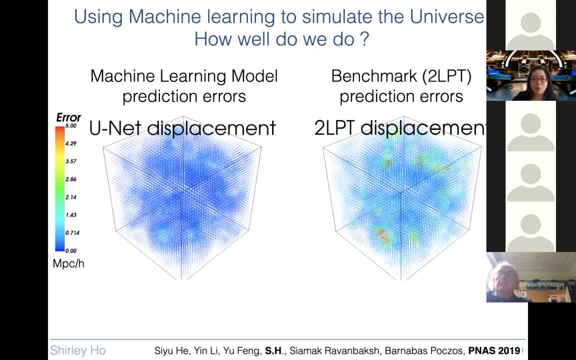 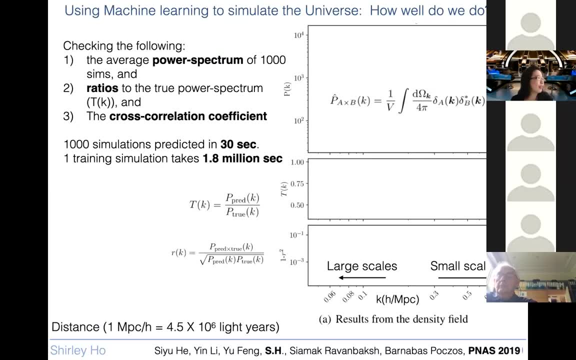 maximum for both. it's the unit model performs 10 times better. let's check a little bit more, and you know, quantitatively, not just qualitatively. we check the following: the power spectrum of a thousand simulations, the ratio so these thousand simulations are predicted using. 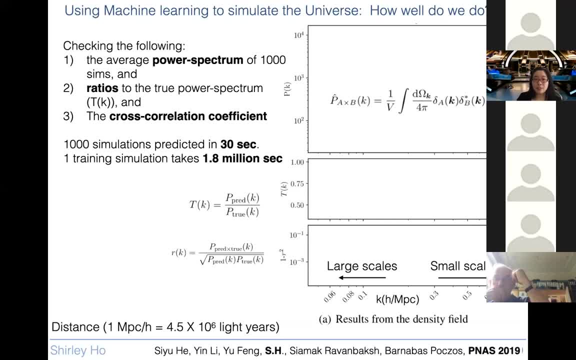 machine learning and these thousand simulations predicted in 30 seconds. why i want to remind you that you know we can, for each training simulations, if you want the end body ones, it's 1.8 million second and we have checked and the ratio of the true power spectrum from you know, either the 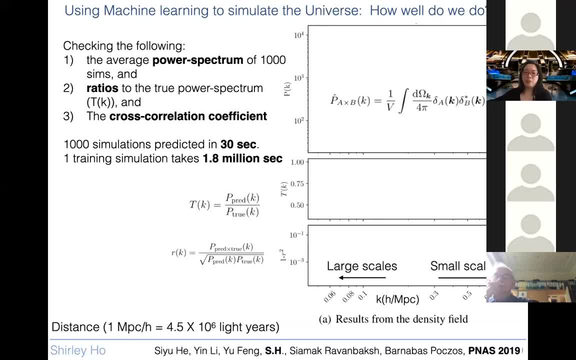 machine learning or the benchmark and the correlation coefficients. i'll show the equations next to the plot. i hope people can see the large goes to the left, small goes to the right, because it's a lot easier to get together and all these things are done in the same way. 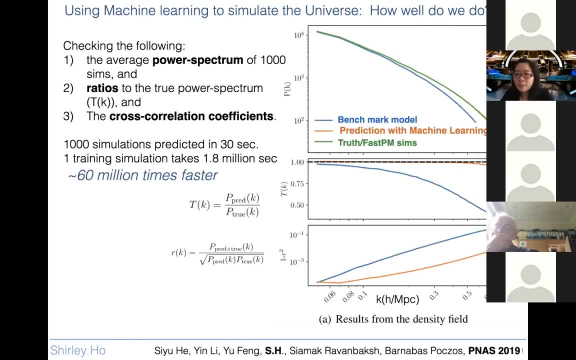 because the measurement model is very well structured. so you can see that the measurement model is very well structured and you can see that it's very easy to mix up. you know the ratio because it's um easy to mix up sometimes and you can see that or you might not be able to. 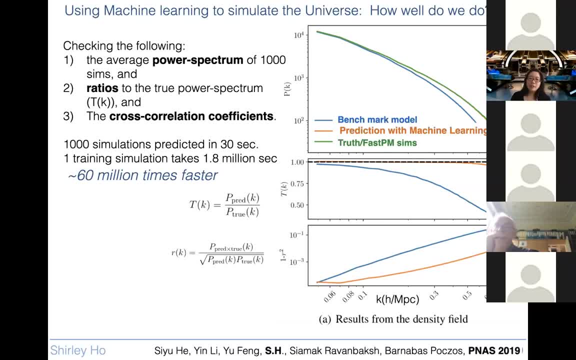 see, sometimes the benchmark model is doing pretty well. actually, if you look at it it's the blue line and you can see it's following the prediction. i mean the truth or the fast pm simulations pretty well. but if you look at the prediction of machine learning on the top you can barely see the orange. 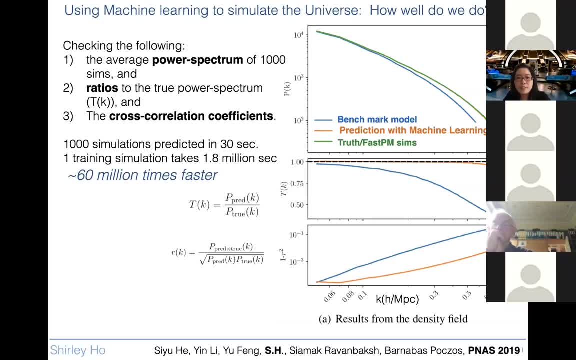 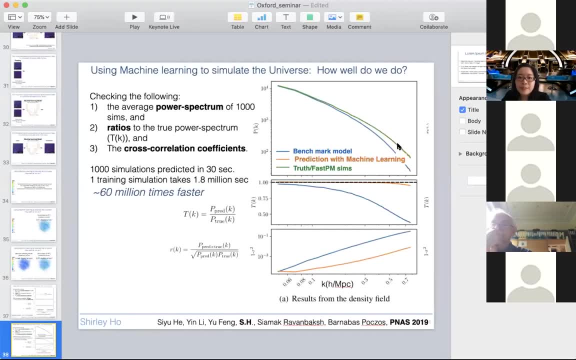 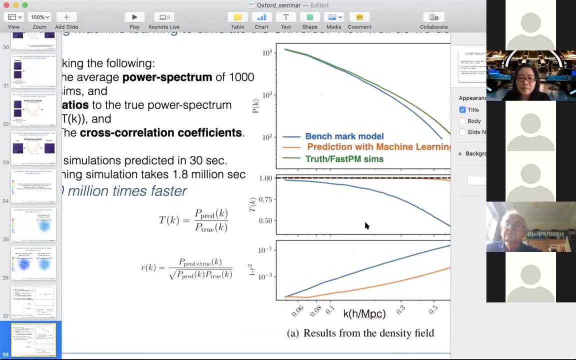 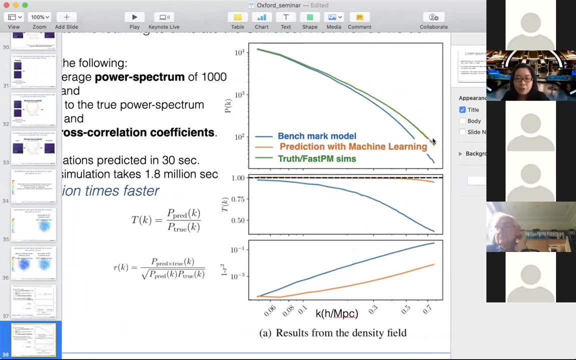 green line is the truth and i know you guys can see it properly and zoom right now refuses to let me find my arrow. can you guys see it better this way? so, basically, the orange line is way hidden by the green line, which is the truth, and orange is the prediction, with the 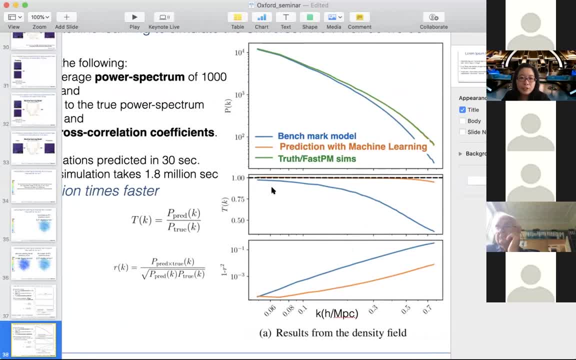 machine learning. if you look at the ratios you can see the transfer function between the power spectrum from either the benchmark or the prediction to the truth. here again machine learning is doing really well compared to the benchmark model. that also runs really fast, and also the correlation coefficient, which is important. 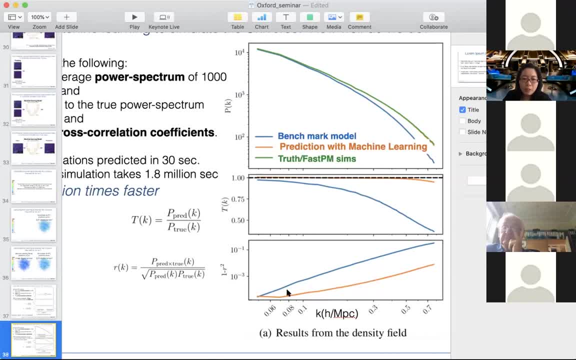 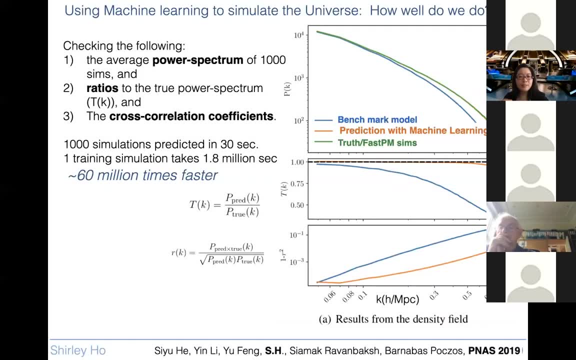 the machinery has much smaller error. this is one minus r squared, so lower is better. it's sort of equivalent to the area power spectrum here, and also it is 16 meters and it's a little bit smaller than the. this is a wide area and it will never be a billion times. 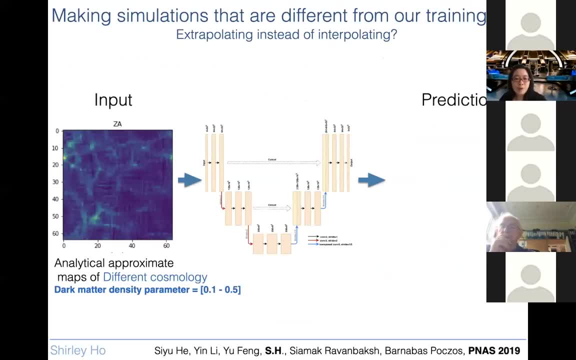 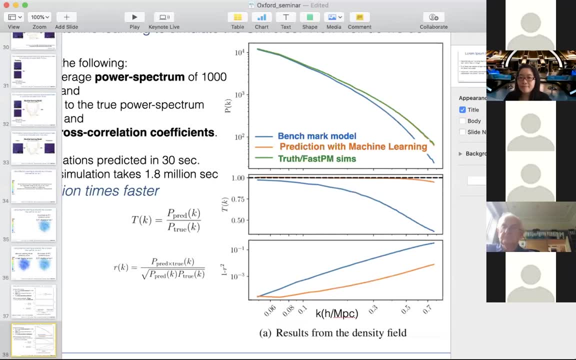 faster, so that's good. so let me just pause and see if there's any questions, questions, questions. no, everyone knows about my awesome work. no questions, real quick. uh, what was the loss function for you? the last function is very simple, it's just msf between the displacement in the prediction and the truth. 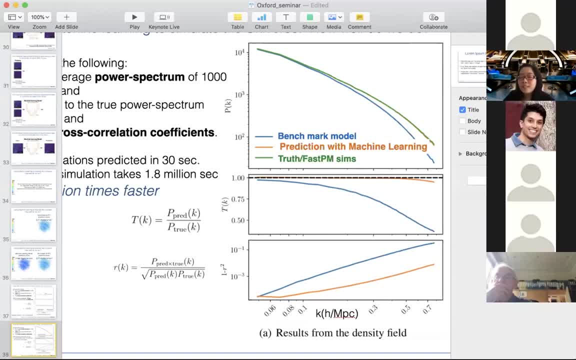 Okay, have you played around with that at all? We did not at that point, but we did play with it afterwards And then, realizing that you know, at first I thought we should do some interesting physically driven constraints in the loss function or regularization for the machine learning crowd here. 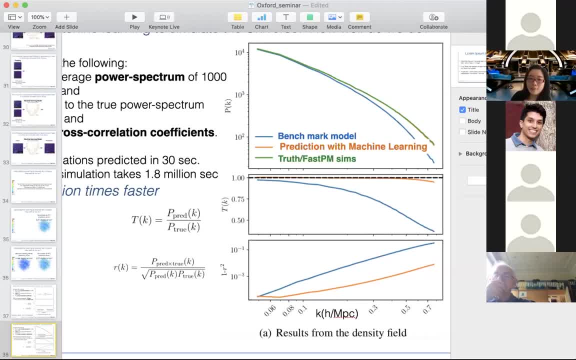 And realizing that, you know, this MSC itself already contained the power spectrum, sort of automatically right, Because it's comparing whether the displacement field are doing really well, whether it should be where it's supposed to be, And so we could do a little bit more. 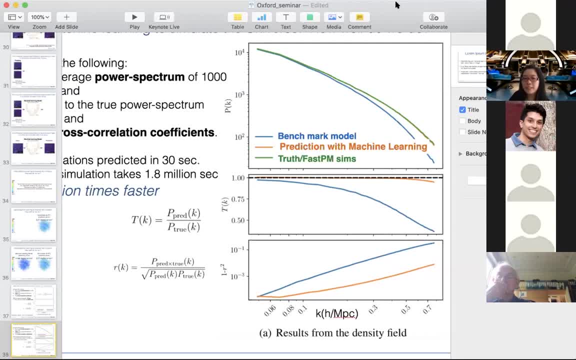 but we haven't done a lot more in playing with the loss function. This is like off the box. We ran with a unit, we tuned the unit parameters, but we didn't tinker with the loss function much. Any other questions? Yeah, good question. 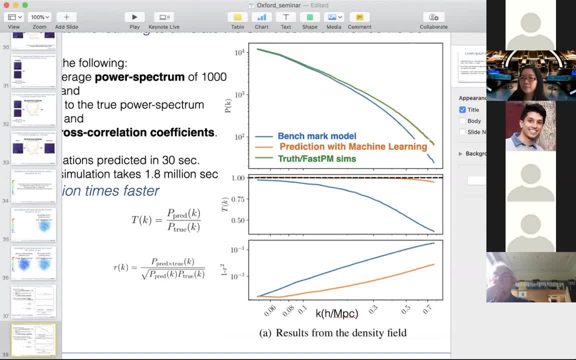 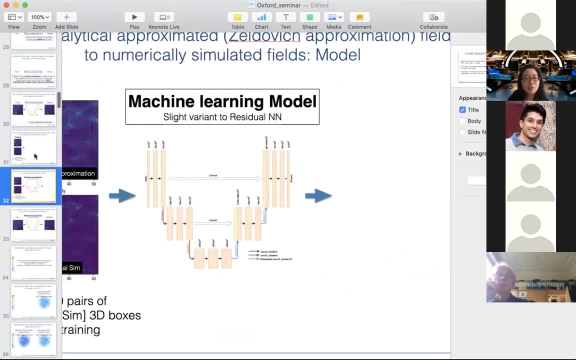 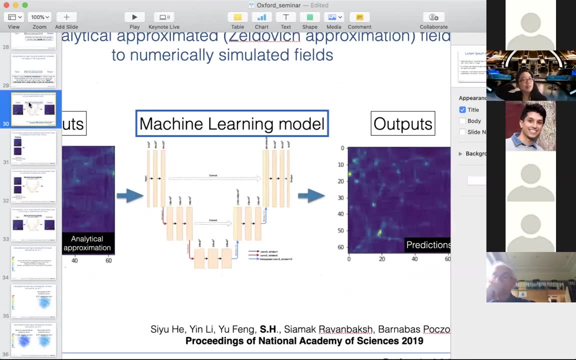 Why did you choose the unit over, for example, Hamiltonian flows or other generating flow networks? Yeah, so it's funny. So at that point, unit was not so popular. yet. This is remind you guys. this work started more or less 2016, 17,. 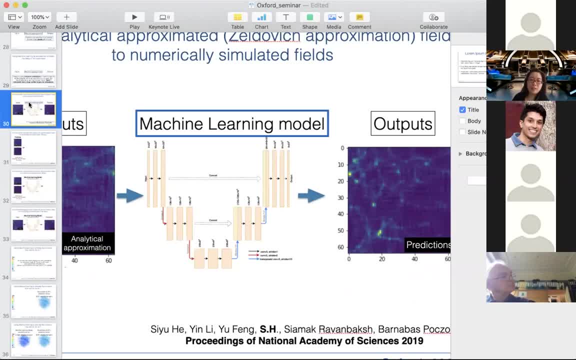 actually probably 16,, 17,- yeah, 17,- or maybe even a little bit talked about at 17. And I think unit was doing really well in the medical imaging field And we thought it was quite interesting to try it out. 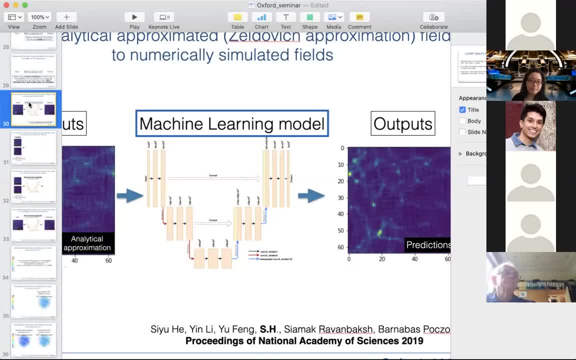 We tried out, it worked and we didn't actually move to a different architecture. So it was sort of luck at same time, but I believe there's some physical insights that drove us afterwards to think about. you know, these are different scale convolution. 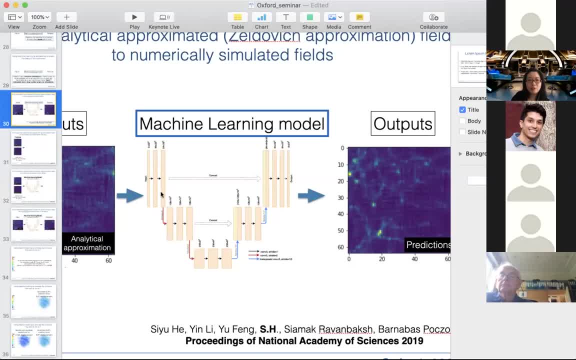 and the fact that it's concatenation, which means we can just take the info from the input, from the input, directly to the output, when you know the large scale is supposed to be correct. I think there's some analytical insight that we didn't expect to be that important. 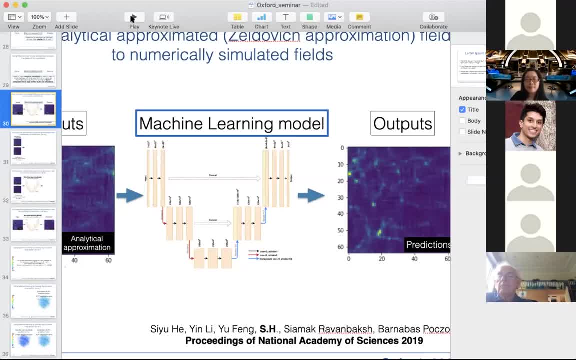 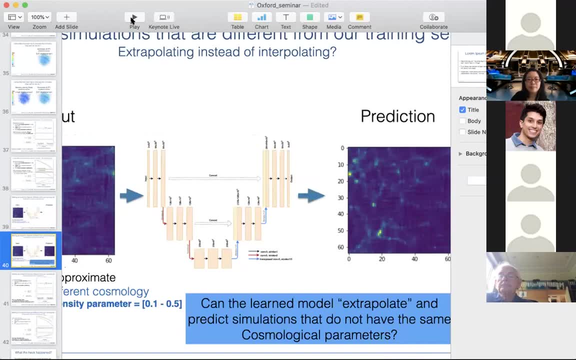 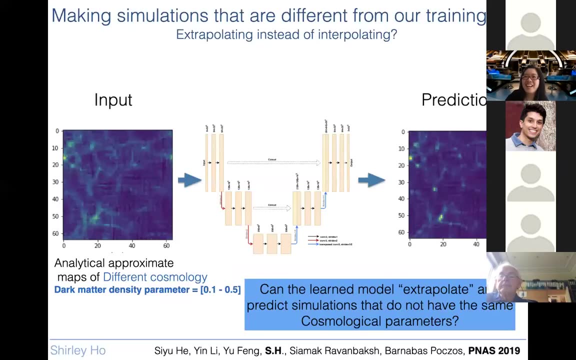 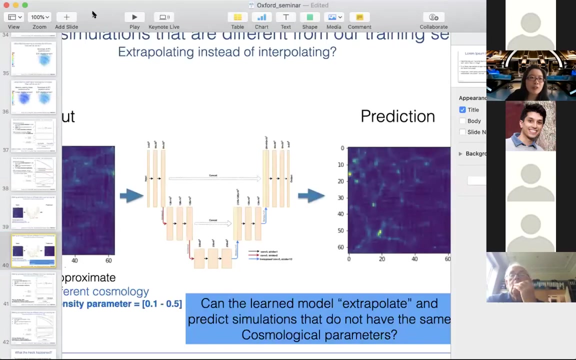 but it worked well. Other questions? If not, I'll keep going quickly so we don't stay too long, because people will fall asleep. Oh wow, I just realized, if I do that soon, we'll actually just show me all your faces. 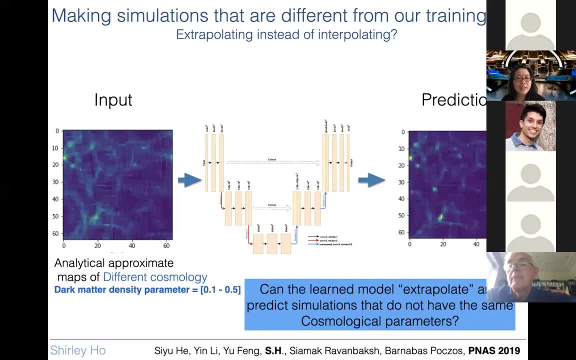 which is great, but it will block my screen, And so we thought, okay, so there's just one more thing, right? We thought we can right now learn from a bunch of simulations. It can predict simulations of the same parameters, which is useful. 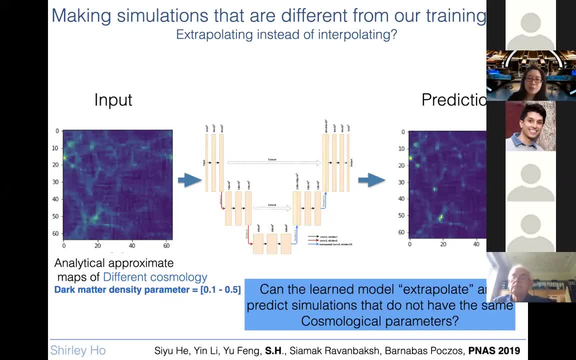 You know you can make covariance matrices very fast, but it doesn't really do what I claim to do. I claim to do is that we need to have different cosmological parameters for these simulations And do it really fast Right now, what I just gave you earlier. 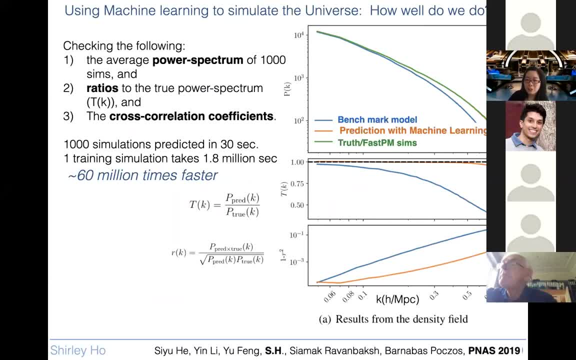 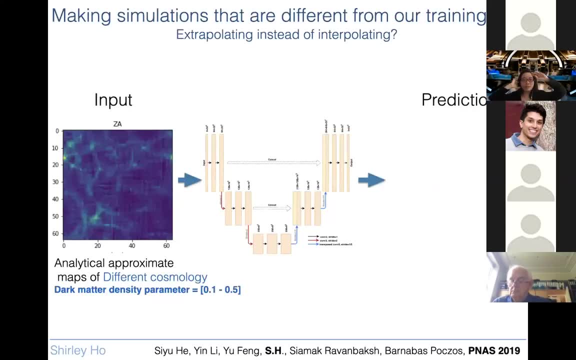 was basically predicting the same simulation, but 16 million times faster, which is cool, but not as good as what we wanted, And so we tried to see something, whether it will happen, mostly because the students thought: why don't we try? 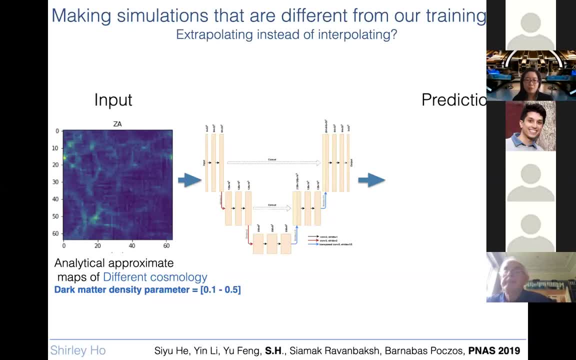 We input different analytical approximate maps of different cosmology where the dark matter density parameter are different. So omega matter is like 0.1, 0.2,, 0.4,, 0.5, even try 0.9.. 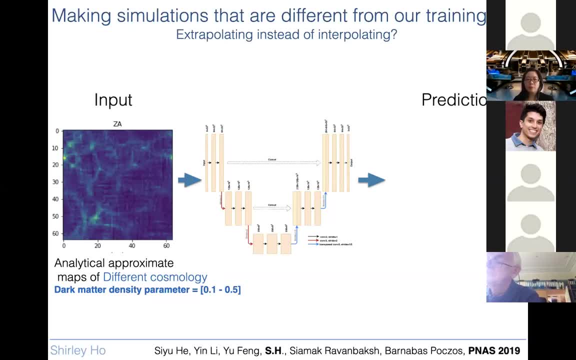 Crazy ideas And we did not retrain the network, which basically means the network has only seen omega matter equals 0.3 and see what happens. Can the learn model extrapolate a little bit and predict simulations that do not have the same cosmological parameters? 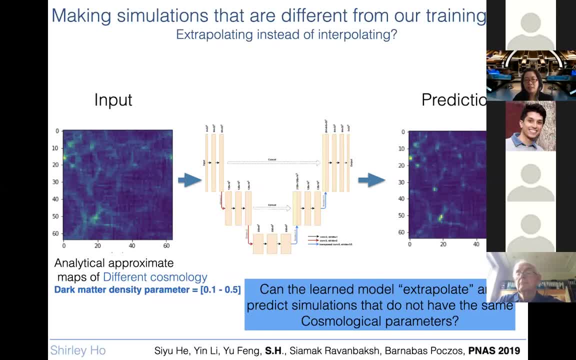 The reason being. you know, don't forget, the analytical approximate still has all the large scales, information correct, right, But all the small scale interactions maybe it doesn't have as strong a dependence- Maybe it does- of the cosmology parameters. 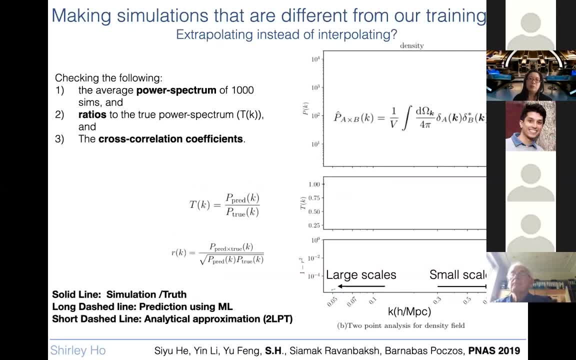 so let's see what happens. So we did that. We check the following for difference: cosmological parameters for omega matter, for example. we still check the average power spectrum of a thousand production seams, The ratios of spear power spectrum, the area power spectrum which is one minus R squared. coz square. Yeah Yeah, Yeehaw, Yeehaw, yeehaw, yeehaw for a combination of the bit Orleans, to the distance between each number of fractions. That was this we kind of like versus what. 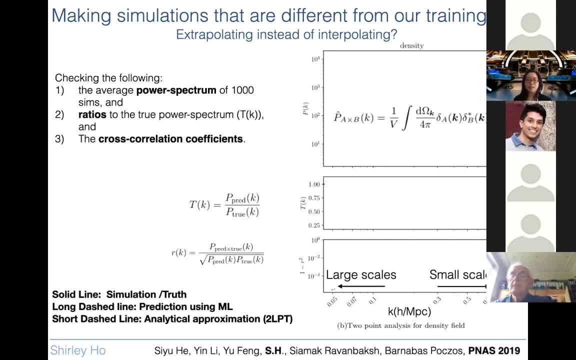 correlation coefficients. Here it's a little bit more complex. plot: The solid line is the simulation, The long dashed line is the prediction with machine learning. The short dashed line is the benchmark analytical approximation, which runs fast. So let's see what happened. I don't know if 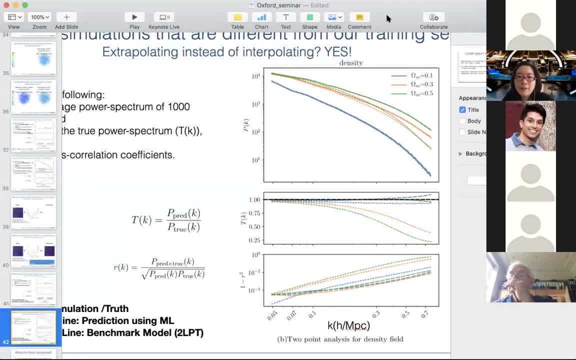 you guys can see, but let me get back out again so you can see a little better, with, hopefully, some guidance on my mouse. The solid line is what we want, because that's the truth. There are three different colors here for three different cosmological parameters for same cosmological. 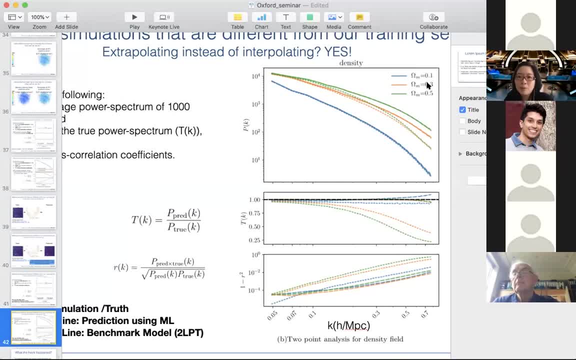 parameters for three different values: Omega matters 0.1, 0.3, 0.5.. Omega matters- 0.3 is what our training was at, So you expect it to do very well And you can see that you basically do not. 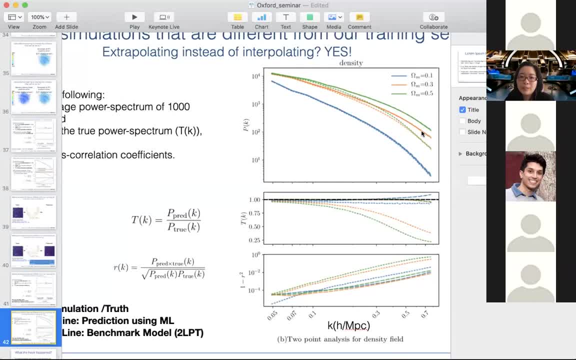 see the long dashed line anywhere for orange because it's under the solid line And surprisingly, it is nearly the same for omega. matter equals 0.5 and 0.1.. The long dashed line is well hidden under the solid line, Or you can look at the ratios here. 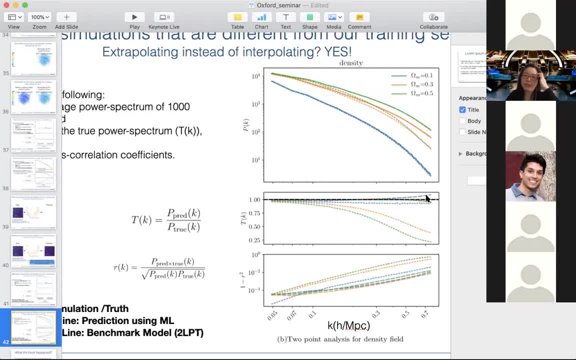 And you can see, basically the error is very small at about k equals to 0.7.. And, honestly, this plot has improved since we trained it with a much more complex simulations And it's in percent level without us retraining the network. So it's kind of interesting. 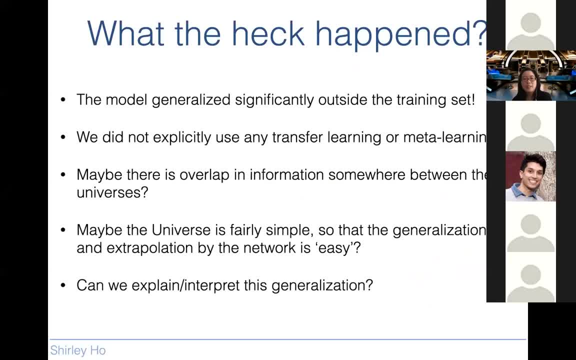 Rethoughts What the heck happened. The model generalized significantly outside the training set. We did not explicitly use any transfer learning or meta learning skills that people tend to do. You train something and you retrain it and do something different. Maybe there's an overlap. 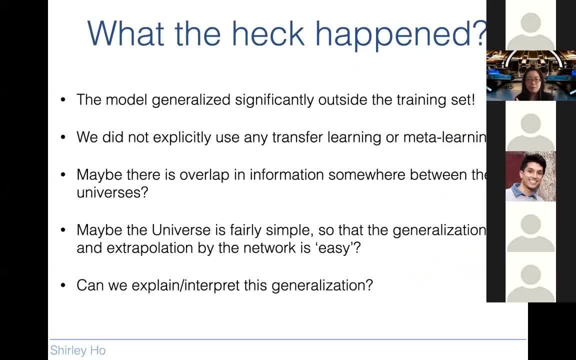 or information somewhere between these universes, which is also possible. Maybe the universe is fairly simple, So the generalization, extrapolation by the network is easy. Can we explain or interpret that? So I would usually go into the training set. I would usually go into the training set, I would. 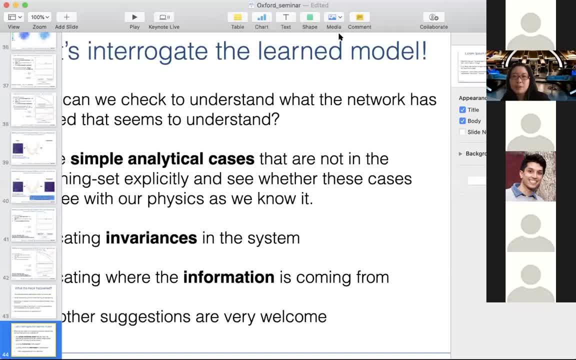 usually go into interrogating this model with this afterwards, But I feel like with this crowd, I might just want to ask what people think happened, To give you a bit more hints. it also works with AS, not just Omega matter. Let's see what people think. Suggestions, what happened? 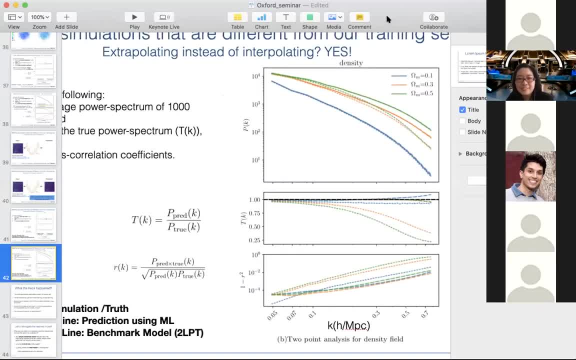 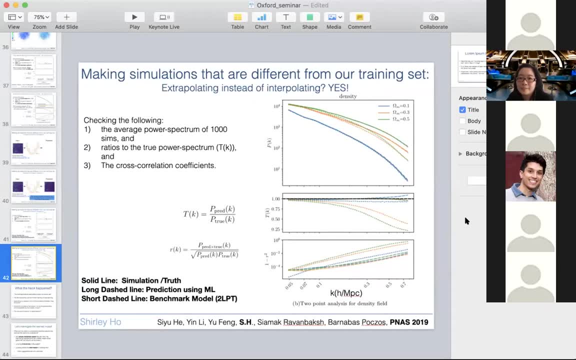 I can go back to this slide. Okay, So we have a little bit of a. So we're trying to network with one set of cosmology. Now we input different cosmology. So we're trying to network with one set of cosmology, Now we input different cosmology. 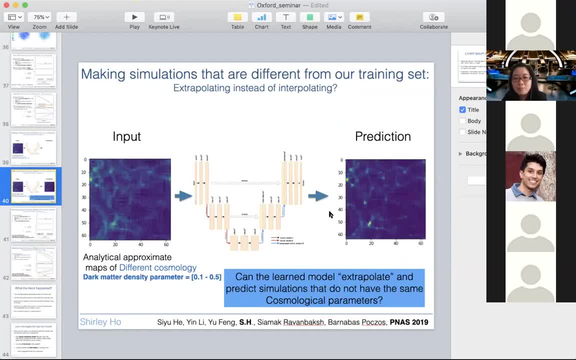 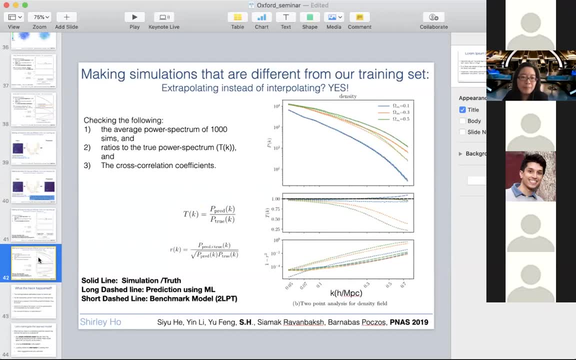 cosmology parameters, approximate maps, it still predicts basically the correct outputs. so it's kind of interesting, right? i'll leave this as a mystery for people in the interest of time, because i want to tell you something further that i didn't usually talk about, so i'm going to skip. 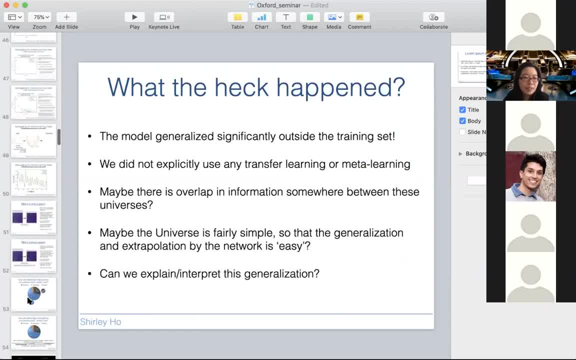 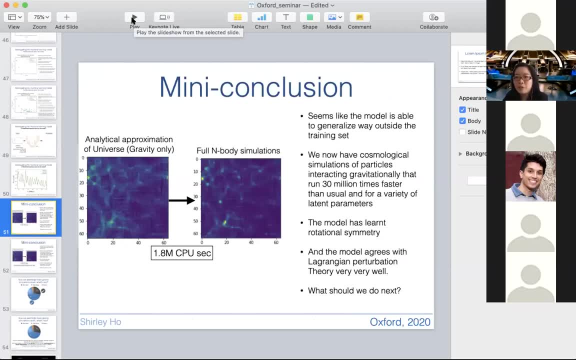 forward to try to explain this a little bit more and show you the meaning conclusion before i show you something else, unless we really want to know what happened, i mean we don't have the true answer yet. also, this is just investigation, what we have learned since. but i'm going to skip that part. 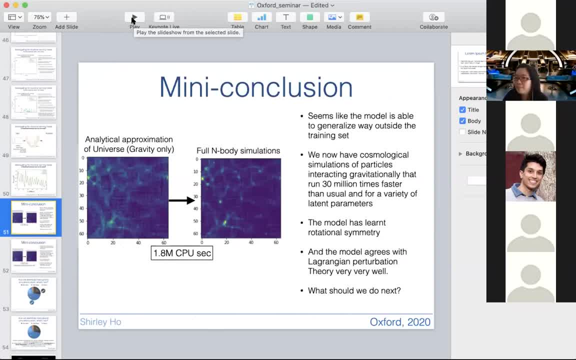 because um, seems like people can't come used to over it. you can come back to me later on too, so the mini conclusion here, which i think is kind of cool to know. sorry about that, let me just make it better. seems like the model is able to generalize way outside. 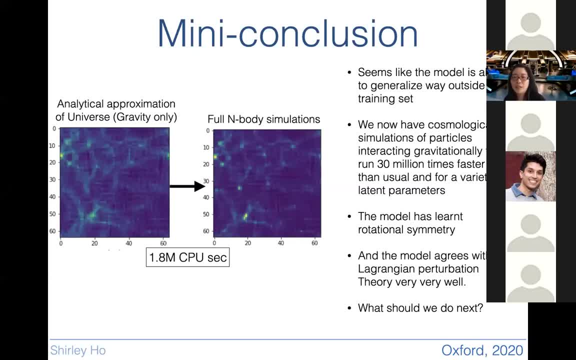 the training set. we have now cosmological simulations, particle interaction graphically that runs 30 million times faster than usual or 60 million times, doesn't matter. it depends a little bit on how much training you use and is in which simulations you use as trains of comparison and for a variety of latent cosmological parameters. um a little bit that you 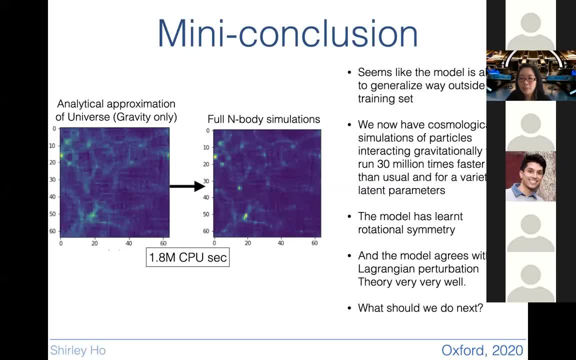 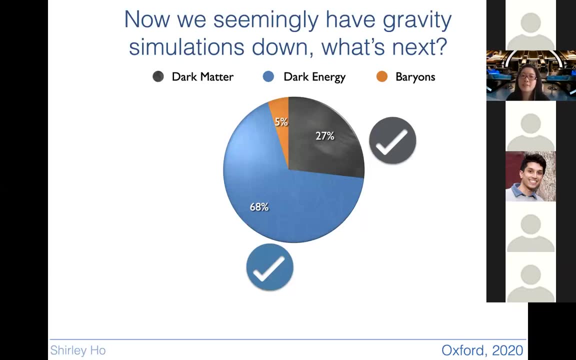 would know that the model actually has learned rotational symmetry. and the model agrees very well with perturbation theory. this is something we learned later. what should we do next? right, so we seem to have got the gravity simulations down, at least for omega matter, and as we've, 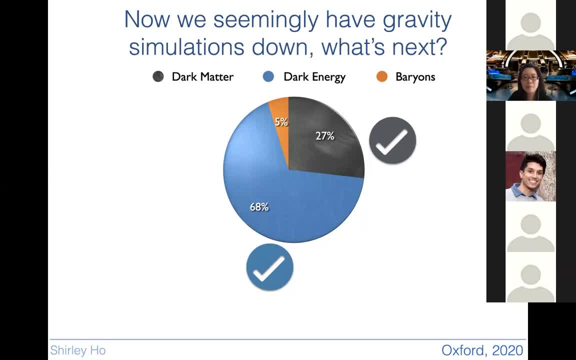 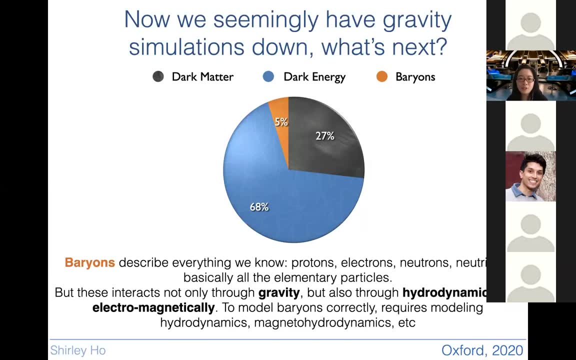 actually been looking at sigma 8 and other parameters right now. so the next part is the harder part. the baryons describe everything we know- the protons, the electrons, neutrons- and translate all the elementary particles. but they interact not only through gravity but also through. 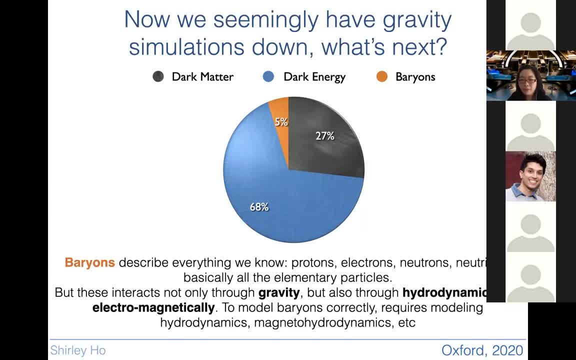 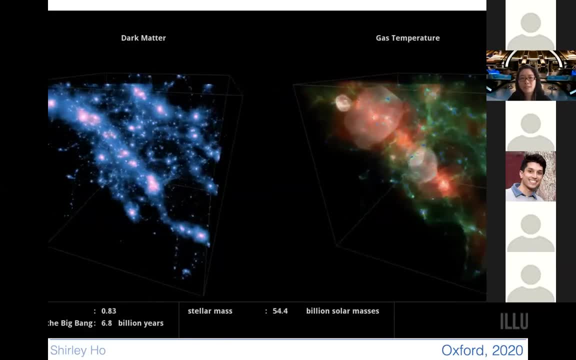 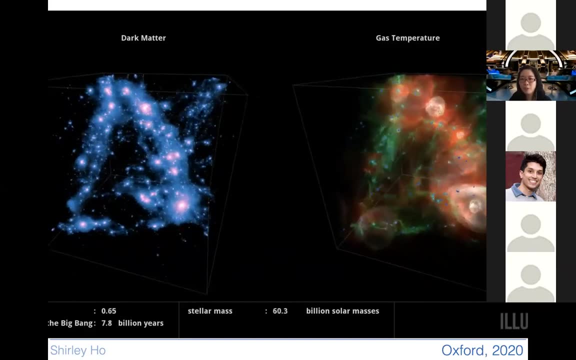 hydrodynamics electromagnetically. so to model baryons is tricky. remember the picture we showed the simulations: on the left is the dark matter, on the right is the gas temperature. the dark matter looked horribly simpler than the gas temperature if you look at this. but we wanted 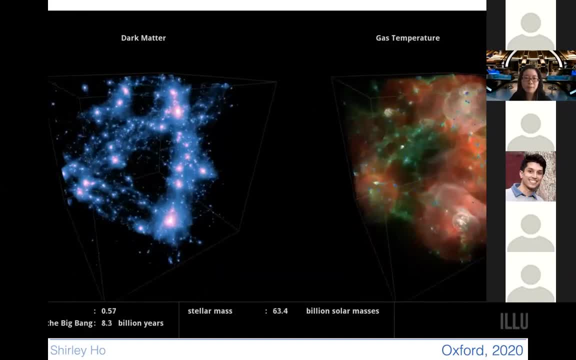 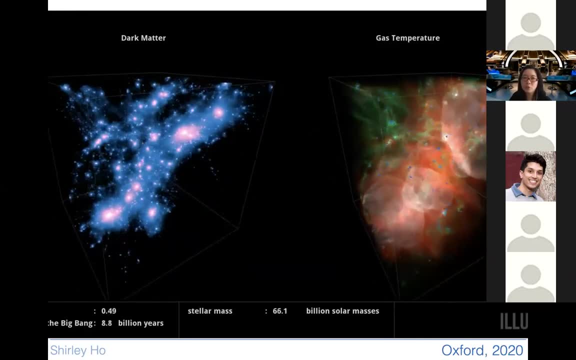 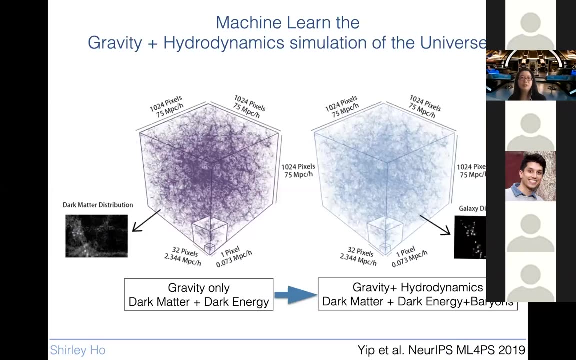 to simulate the baryons, which is on the right, much better and much faster, and the simulations on the right took 30 million cpu hours to generate, so a thousand eight hundred cpu seconds if i did it right. so i tried to do this. machine learned the gravity plus hydrodynamic simulation of 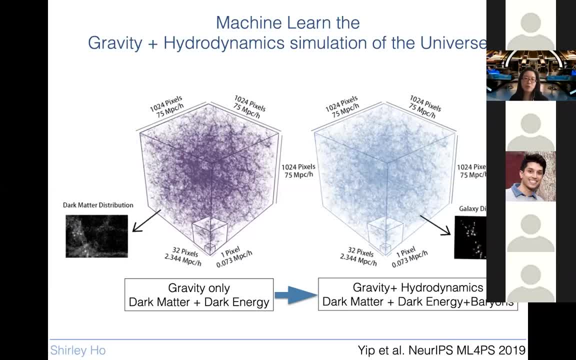 the universe. how do we do that? we want to go from. you know now we can generate gravity simulations super fast, like milliseconds. can i go from this gravity only simulations to gravity plus hydro to get the galaxy distribution correct? so that's the first step. it was published at: 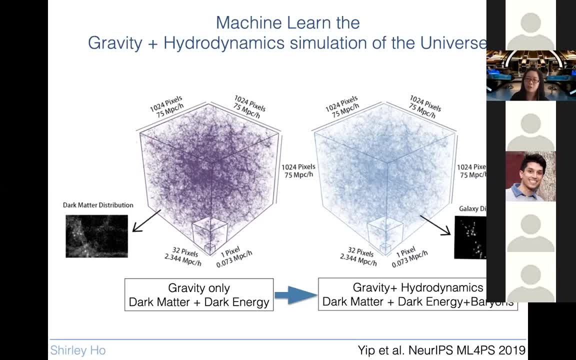 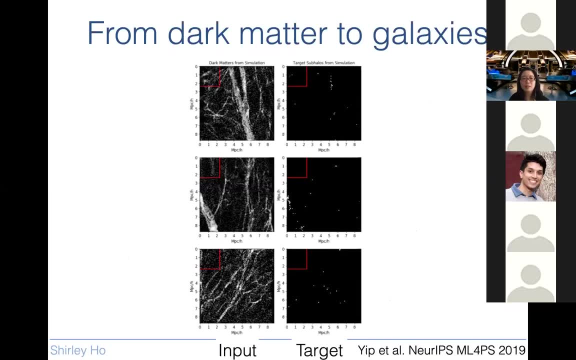 nerfs, which is this um, machine learning, but one of the biggest machine learning conference. i think 14 000 people showed up when we went last year in december. so what we did is that on the left hand side is this: this left column is a dark matter density field just projected in 2d so that not 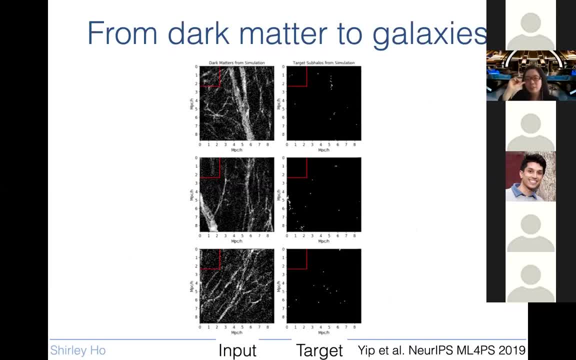 for the interest, 2d slice, and on the right hand side is this target distribution of galaxies and you can see that you can barely see these little dots there. it's actually quite hard, and not that many galaxies are there with so many more dark matter particles on the left. so it turns out to 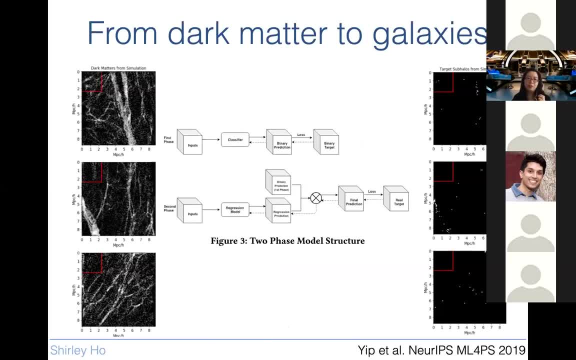 be not so simple. it's actually surprisingly harder project than the last one i described to you, but the idea is simple. it's similar. you have maps on the left and you have maps on the right. the maps on the left is describing a field that you want. you already have very easily accessible. 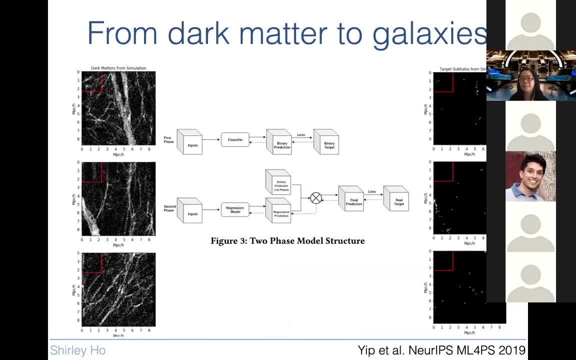 you can create easily. the maps on the right takes, you know, 30 million cpu hours to create one. you know little cube, so you want to sort of skip that procedure. and because it takes 30 million cpu hours to make this one simulation, we only got one as training set. no 10, no 10.. 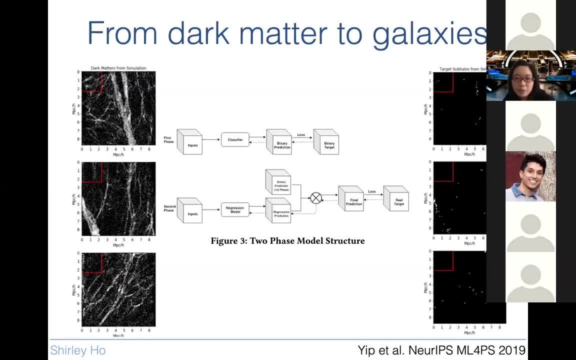 thousand, just one. and here's the model structure we use. we use a two-phase model structure, which means that two steps. the first step basically figure out whether there is a galaxy or not, so it becomes a binary projection. it's much easier to do. and the second step is if there is a galaxy. 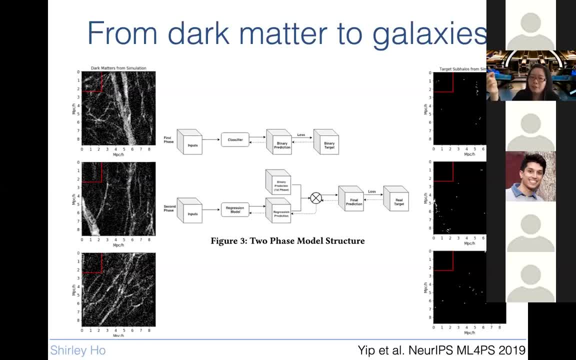 in that little pixel or foxo- how many are there? which the second part is very similar to our unit architecture, as you see in the bottom. it's nearly the same, but we decide to change a few things. um, there are reasons why we do it a certain ways, but we can talk about in details later. 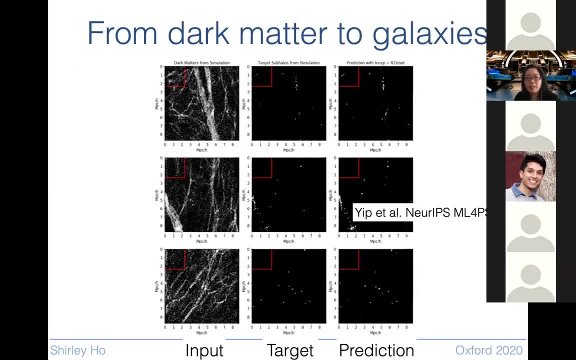 and now you can see a prediction on the right hand side and it looked pretty good, at least qualitatively, looked basically the same as target, which is in the middle, and you say, well, okay, it is a picture. so we can do a little better than just pictures. we calculated the power spectrum. 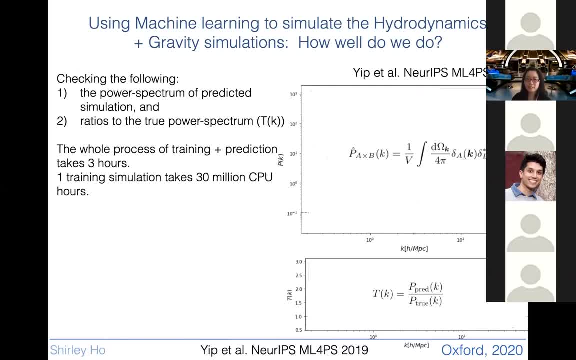 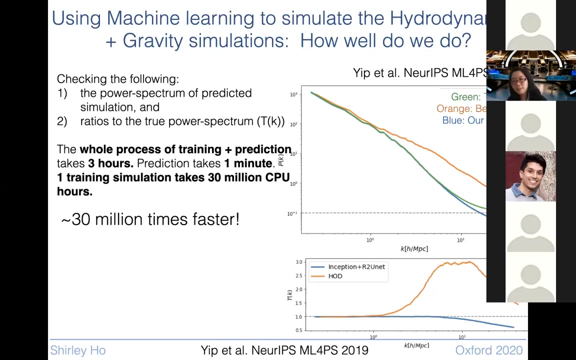 again of the projected stimulation, of the predicted galaxies and we calculate, show you, and maybe the um um shows the true power spectrum. also, the whole process of training and protection takes about and he was like, oh, i wish actually he was doing better and you got to notice that the k for those. 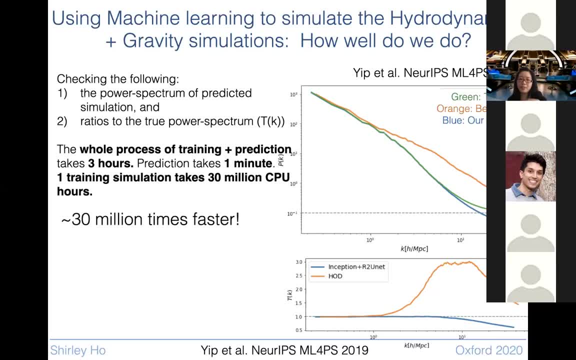 cosmologies in place here. k value here is very high. it goes all the way to a few tens of k and our model is correct to about k equal to seven, maybe six, depending on how you read carefully. on the transfer function, i mean the ratios between the predicted power spectrum to the true power. 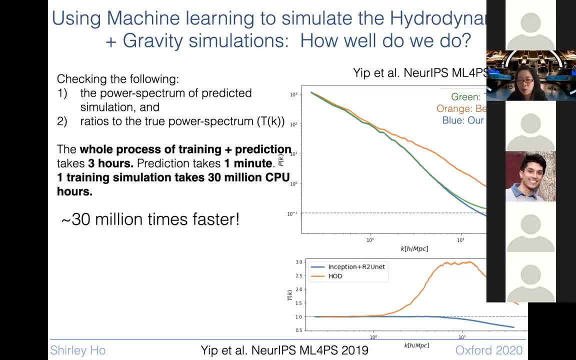 spectrum in the bottom, but you can say it's basically one which is the good number here you want all the way to about seven or six, which is very small scale, and it's 30 million times faster. so we thought that was pretty cool and now we are able to predict where and how many galaxies 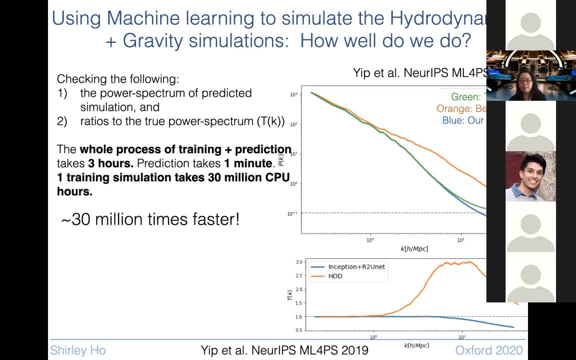 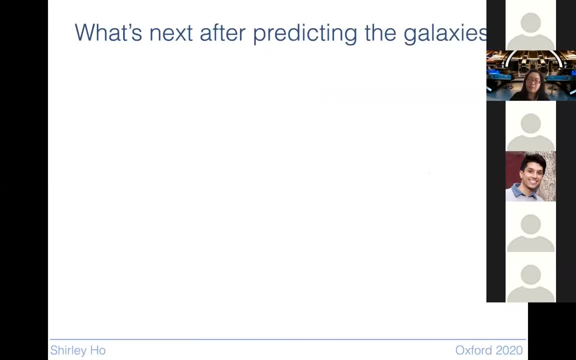 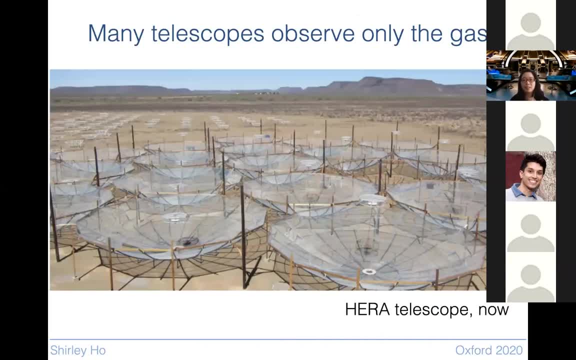 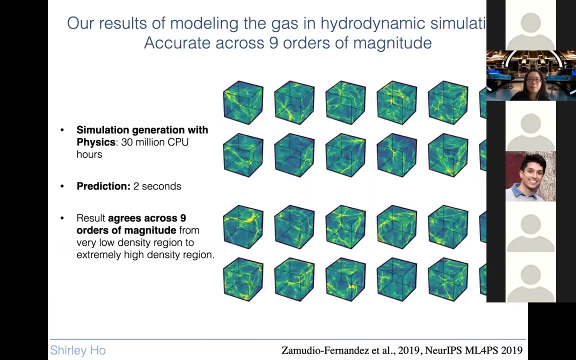 all these. you know various different um, intensive mapping experiments, all this stuff that's coming up. there was um. this project was also conceived at berkeley's, when her telescope is all in rage. but those who don't know about these settlements and experiments? So our results of modern gas and hydrodynamic simulation are accurate across nine orders. 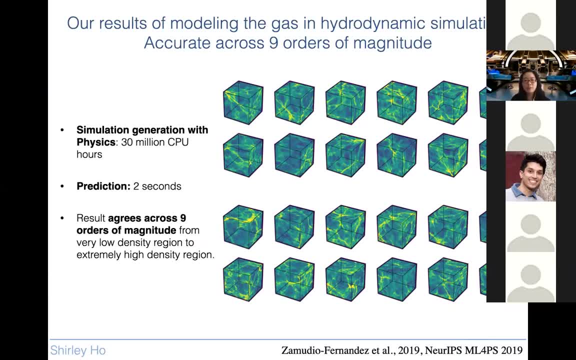 of magnitude compared to the simulations We generate. if you want to generate a simulation which I talked about, this one simulation called Illustrious is 30 million CPU hours to generate it. The predictions took two seconds and on one of these two rows, or two of these rows, are: 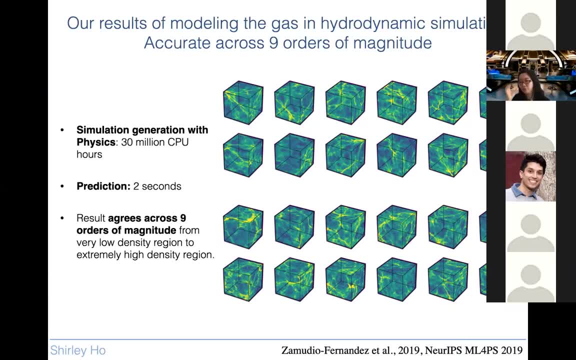 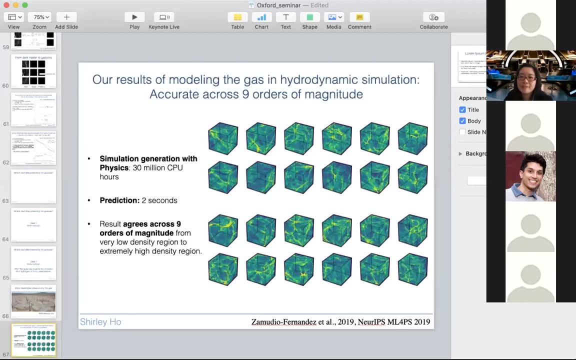 the truth. The other two rows are the simulated universes And I can try to make you tell me which one is the truth. Any suggestions? Let's see Any takers? The bottom is the truth. Any other takers, To be honest, I actually don't remember. 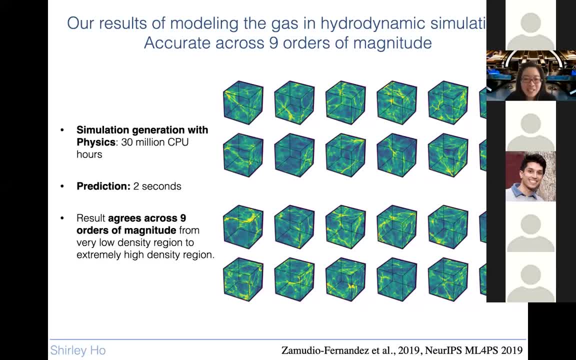 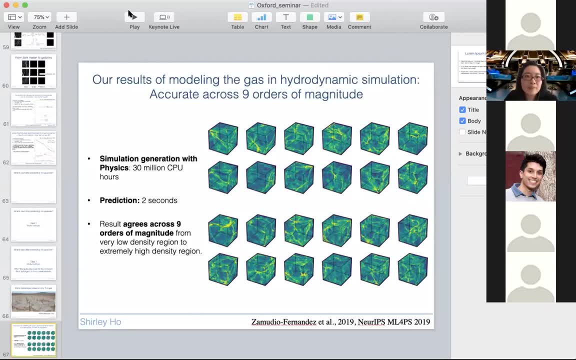 I need to go check my paper For me. I can't tell the difference actually, Because it's quite accurate, and you will see why I say that actually soon. Because quantitative, qualitatively, you can't tell the difference, but qualitatively we. 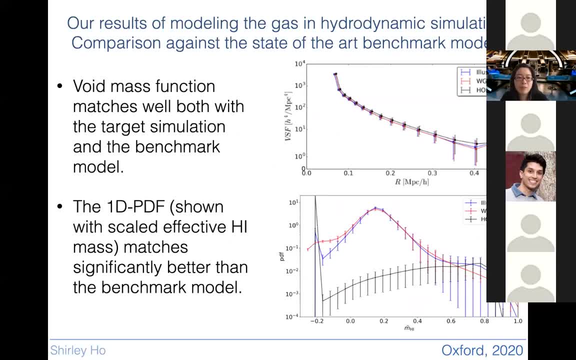 compare the Ford mass function, It matches really well. And the 1D PDF. here the blue line is what we want, The black line is the HOD model. So the HOD model, which is sort of the benchmark model, Paco, which is one of the postdocs on 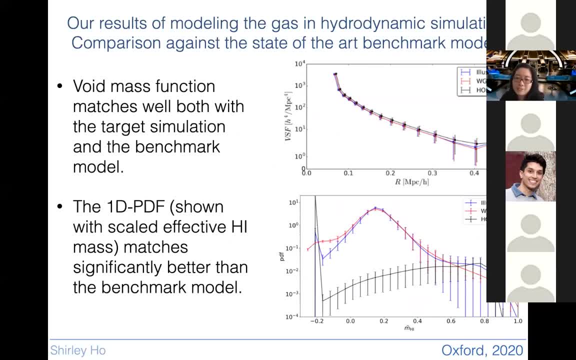 this project sort of pioneered right before this project And it does really well for any heavy galaxies. but it did horribly with sort of low mass filamentary structures, laminar force. but our model is doing really well. Actually the green line is the truth, sorry, the blue line is the truth and the red line 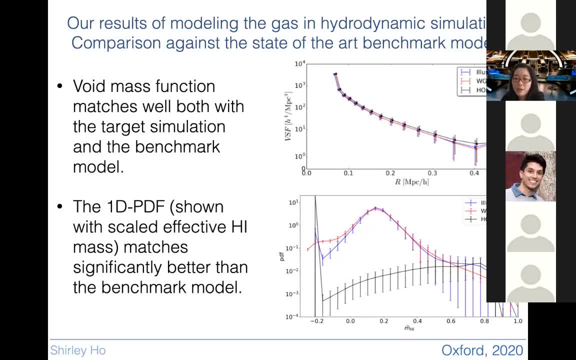 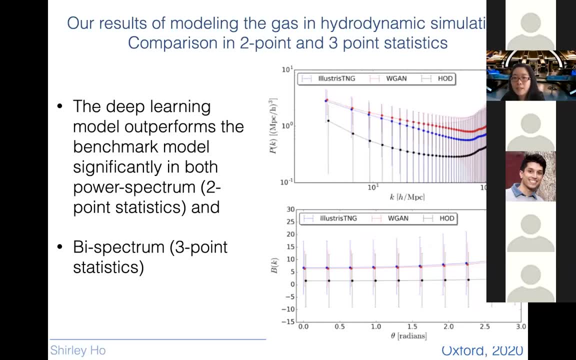 is our predictions, So it matches significantly better than the benchmark model. We also looked at the power spectrum Again. the W again is the red line. It did pretty well with the error bars And also compared to the benchmark, we're way closer. 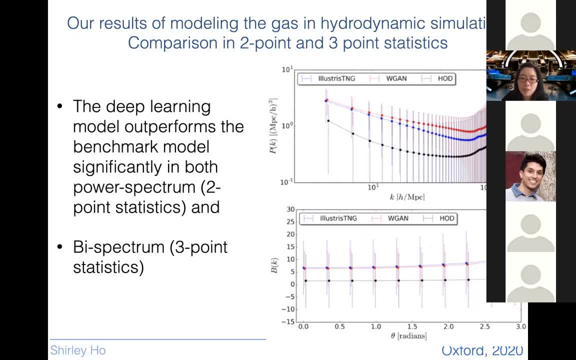 And so is the power spectrum. So is the bi-spectrum, where the bi-spectrum is basically zero with HOD, while we can actually model the bi-spectrum quite well, The gist of it is the red and the blue dots are basically very close to each other. 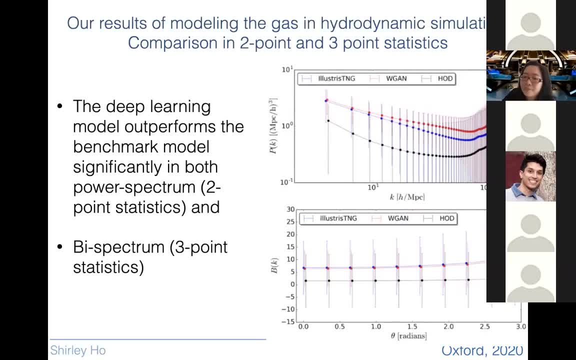 So what have we done so far? Sorry, sorry, Go ahead. Where did the error bars come from? Yeah, this is a very, very good question. So the error bar came from the students running the you know many, many, many test case. 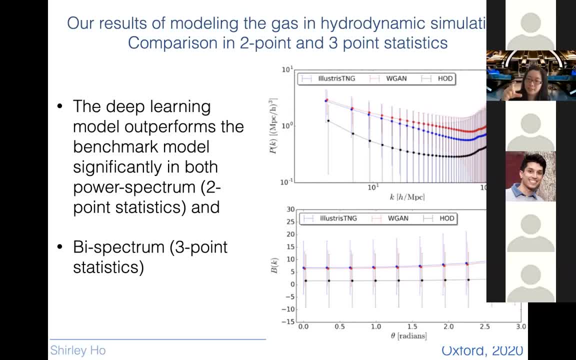 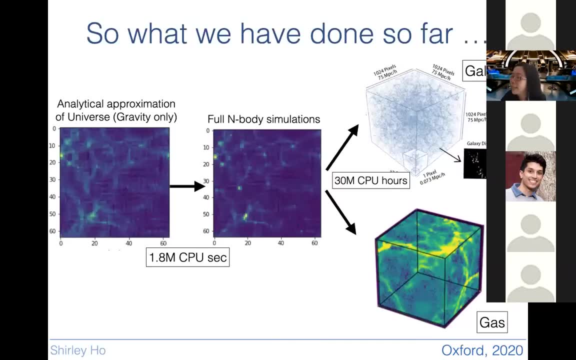 and just looking at the variance of all test cases- and the test cases are very little cubes, Okay, Okay, Let me show you the cubes. And how well calibrated are those? Say that again. How well calibrated are those error bars? Not very well calibrated. 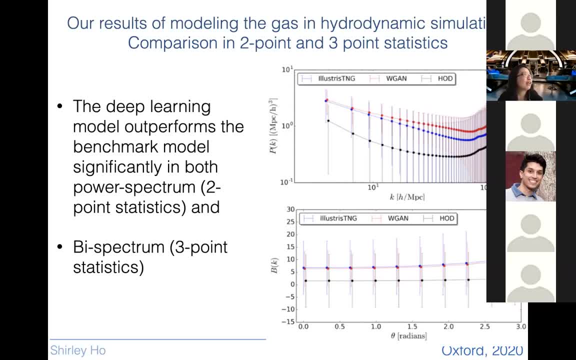 Because I don't think they did like a very careful job in terms of including- you know, possibly- all the errors that you should be including, Like I don't think they even calculate the cost of variance, for example. Okay, 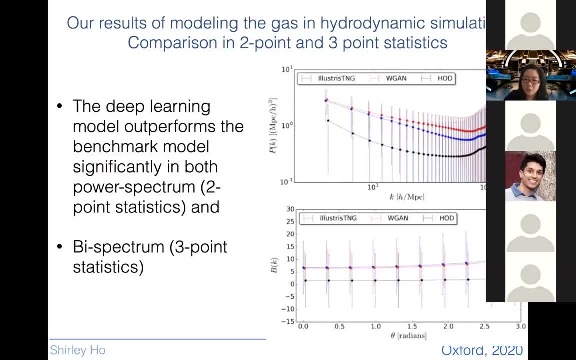 Thank you. Yeah, But you know, this is again. these are students who this work is led by Center for Data Science master students And the four of them we supervise, and I was very impressed that we even get that far. 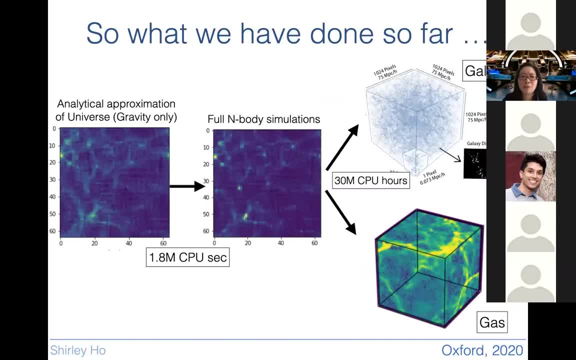 honestly And the master students in machine learning about biospectrum was interesting. So what we have done so far, we had approximate universe in local approximation of universe as input. You can get the full N-body simulations and you can also go and get either the gas or 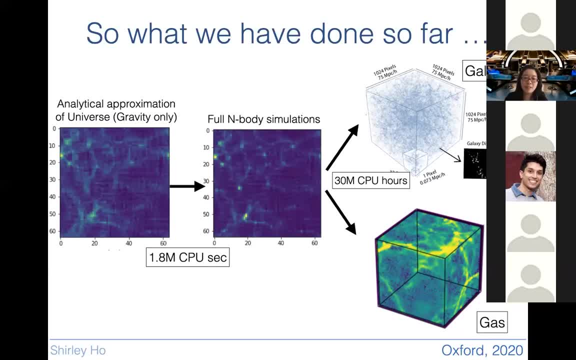 the galaxy distribution And you can see that the time it takes will be, you know, in the millions of CPU seconds, or hours in this case, And now we have the situation where it is .03 seconds to get the full N-body simulations. 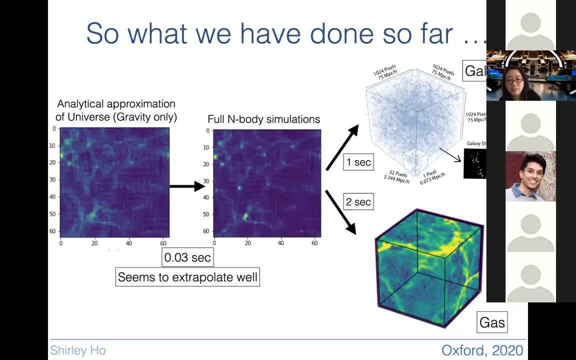 Okay to get the full N-body simulations which extrapolate, well surprisingly, in about one second to predict the galaxy positions, two seconds to predict the gas, the H1 in particular. So I would say I guess I missed Obama, so I. 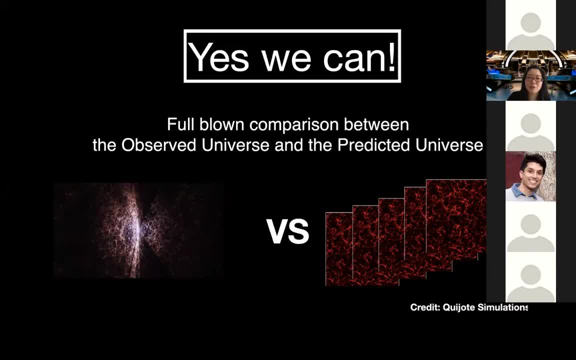 said: yes, we can. There's a full-blown comparison between the observed universe and the predicted universe. It seems like this is a way forward that you can predict. You can basically simulate fully the cosmological universe with both the gas and the galaxy. 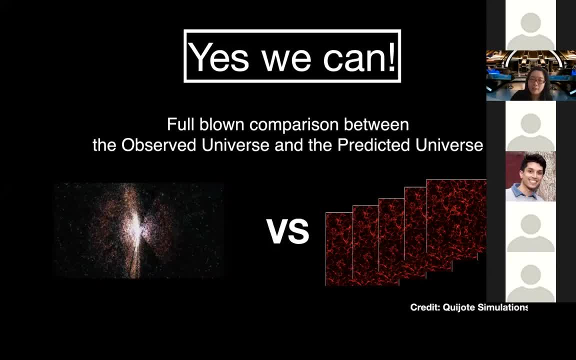 density, number density with very, very little time, And you can compare it with the universe. There's, of course, a little bit more work, right? Because right now we have the number density, galaxies, but we don't yet have colors or shapes We want to do. 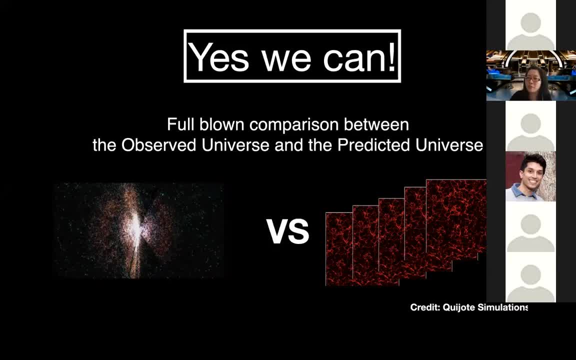 weak-lensing comparisons. We don't yet have the fluxes where you want to use emission-line galaxies, But these are things we're moving forward. I think- the fact that you can even do what it has done so far and shown, I think it's very interesting. 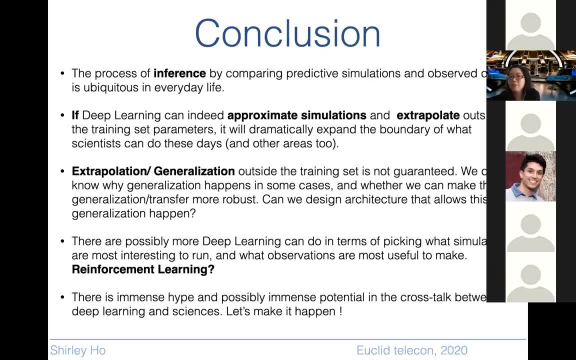 I'll give a quick conclusion, because otherwise it'll take forever. This process of inference that I just described. it's not specific to just cosmology. right, By comparing these predictive simulations and observed universe. in this case, the observable is ubiquitous. 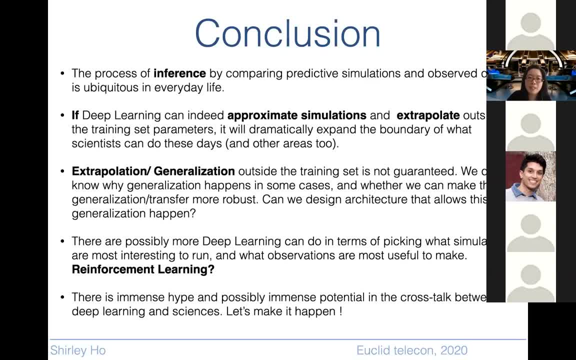 in everyday life, especially for scientists. So if deep learning can indeed approximate simulations and extrapolate outside a training set, it would dramatically expand the boundary of what scientists can do these days, And possibly other areas too, for example self-driving cars. 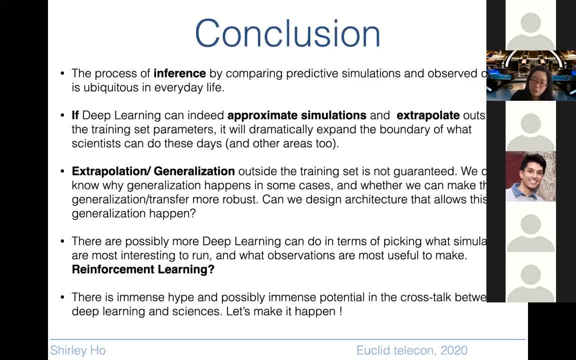 If you can learn what happens when you can train with raining and sunny days. can you actually predict snowy days? I don't know, This might be very difficult. Actually, snowy can do obstruct the signs, Extrapolation or generalization. outside training set is not guaranteed. 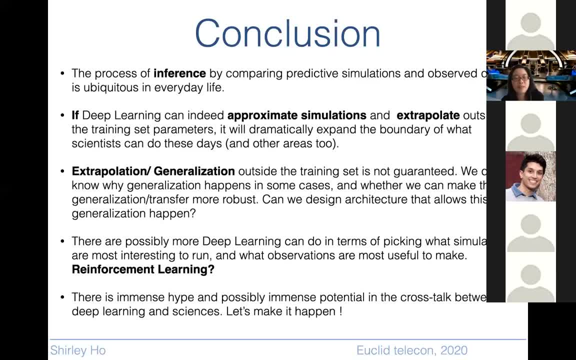 We don't really know why generalization happens in some cases or whether we can make this more robust, this transfer or generalization. Can we design architecture that allows this generalization to happen more naturally? There are probably other machine learning things we can do in terms of picking what. 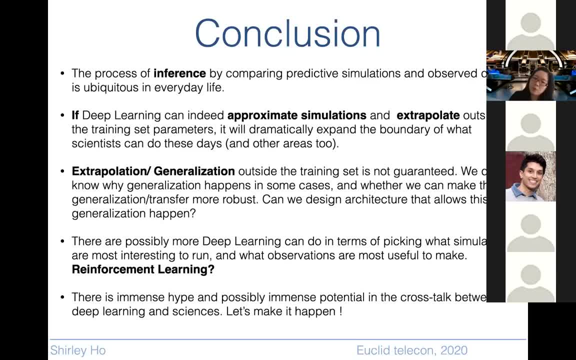 simulations are more interesting to run or what observations are most useful to make, like reinforcement learning would be one interesting idea to look into. There's a lot of hype and possibly a lot of potential in the crosstalk between machine learning and deep learning in sciences, so let's make it happen and thank you. 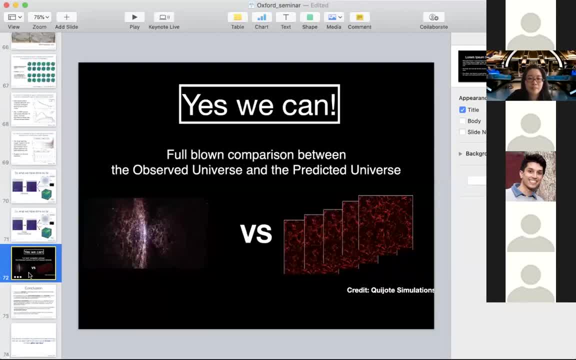 So on this question of extrapolation- I mean in particle physics- we always warn people against using a trained network on data which is outside the sort of the volume of the training data, because presumably the network can do anything it wants with data. 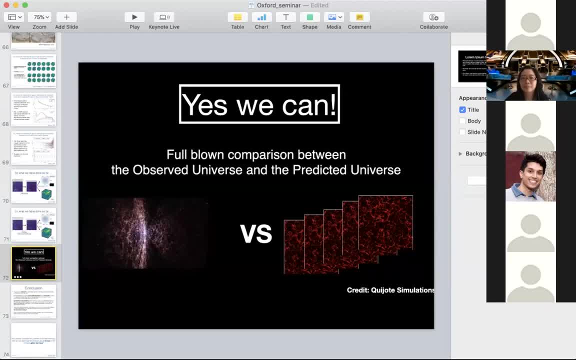 that sort of doesn't occur in the training set Because it won't affect the data, It won't affect the cost. So it sort of sounds unusual that you can actually do it. So are there any hints about what it might be that's doing that for you? 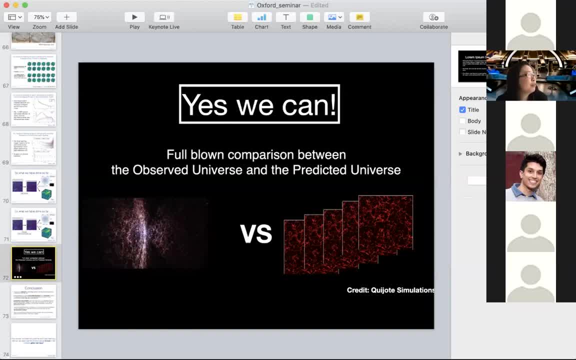 We have a lot of, we actually have a bunch of projects sort in that direction, trying to figure out why it's doing it for us. but we're not the only team that actually can extrapolate. There are a couple other teams that have this interesting situation where let me bring 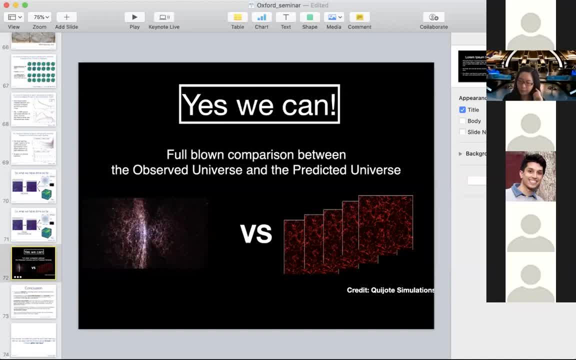 out one. This is a very interesting work by DeepMind, so Peter Patagly and the group are able to simulate the universe- not the universe particle simulations- and they were able to do extremely well in extrapolating and basically generalizing. 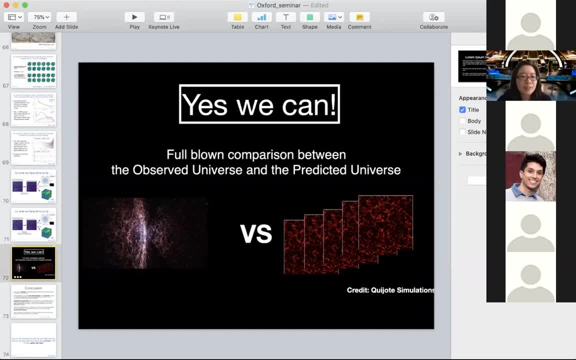 Actually I'm curious if I can show you guys the Twitter page. Actually this will be way too much work. but they were able to generalize to different um, Number of particles, different box sizes, even though they train with one single box. 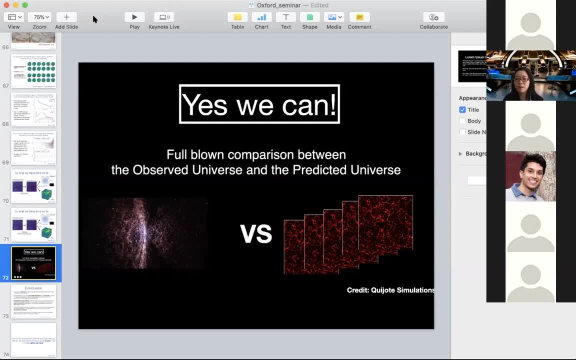 sizes and one single number of total number of particles, and they were able to generalize going further in time steps also, while they train only with one time step. So there are generalizations that's happening, but they have very strong something called inductive bias. 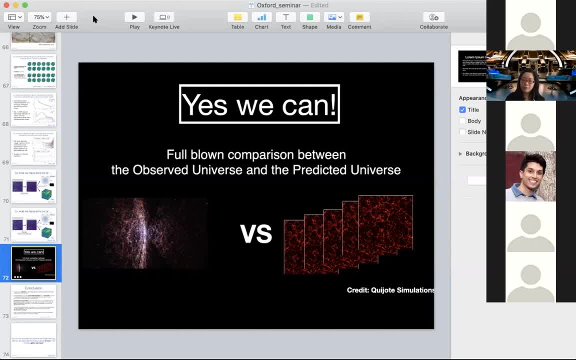 Like in the architecture, they made very strong assumption in the physical by the physical biases. So I think there's some interesting ways that um the machine learning world is discovering is that if you put in interesting constraints from the physics world, you do much better. 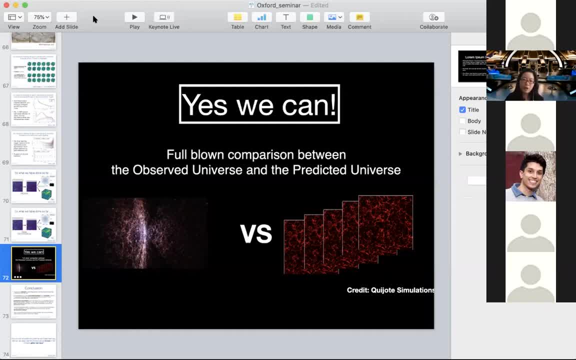 in generalizations. So don't just take you know a network off the shelf and expect generalization. but I think there are situations where it does happen when you put in the right. they call it inductive bias, but basically strong constraint in the architecture based on your data. 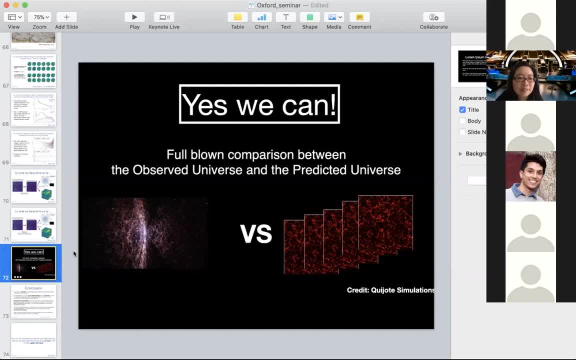 That's usually physical, Okay, Okay, Thanks. It seems you did not use a gauge-equipped neural network, So how did you train it to take into account rotational symmetry? Did you just augment your data set with all rotations, or Yeah, So our data sets were augmented? 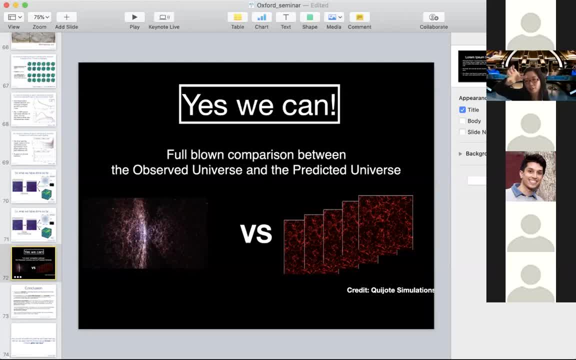